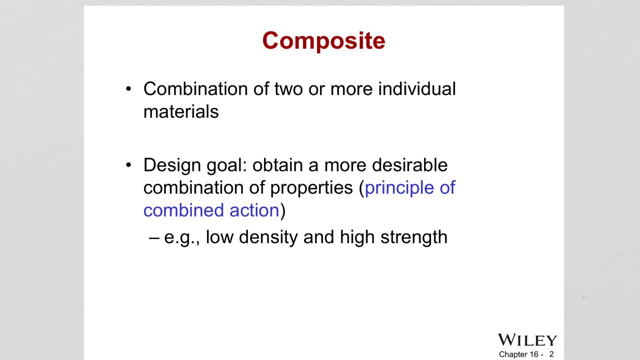 of properties like low density and high strength. so the idea here is to engineer materials to maximize properties of both materials. so examples are like Aerospace applications, like Solar Corrections, uh. structural components, automotive parts, sinks, bathtubs, swimming pools, buildings, bridges. 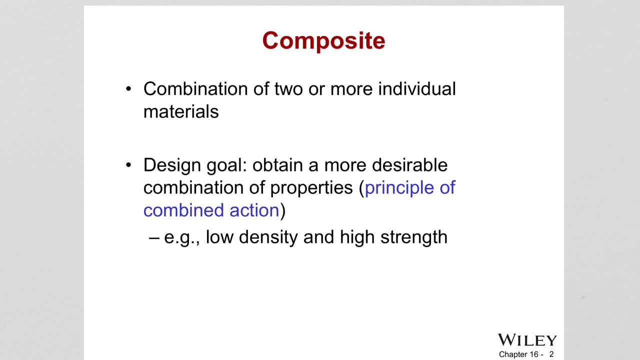 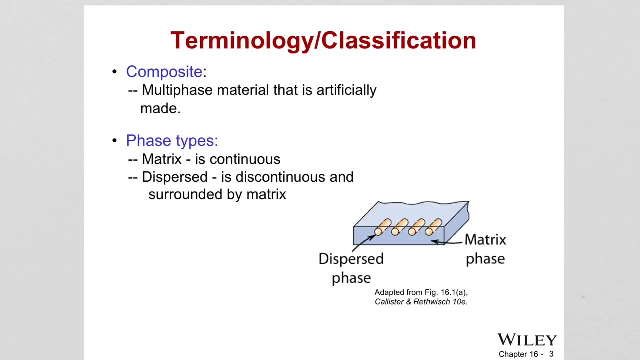 snowboards, golf clubs, finishing pole, fishing poles- So most of the transportation industry and aerospace I mean, and sports goods, these are now currently made of composite materials. So when we say composite, we are talking about artificially made composites. So by intentionally, people are mixing two different types of face. 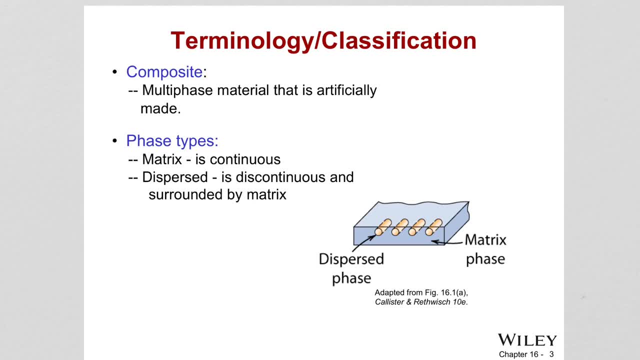 or two different types of materials. So the terminology here is: we have a matrix which is continuous, and it is shown in the image right. Matrix can be a metal, polymer, ceramic. Within that matrix we also have a dispersed face. Okay, so in the dispersed phase, with this discontinuous, like pointy fl cuálKE waveformём diameter is strictly rounding. titled connective BlockingTA is with double diagonal form, factorhallστεaux, Jasper. Within that block you can see sinking two different types: orana path. Then in distance you have category, the base phase And Eastern. 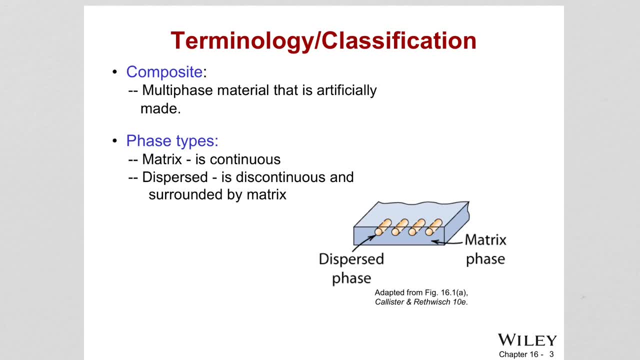 a live pretty will be the upper bound. Forget about these most important too. over S. So it's at the end. of the Fibers and particles. This continuous phase is surrounded by the matrix, So this terminology is not important. You guys need to put this image in your mind. Whenever we say matrix, what does it mean? Or if we say dispersed phase or the fibers, what do we mean? 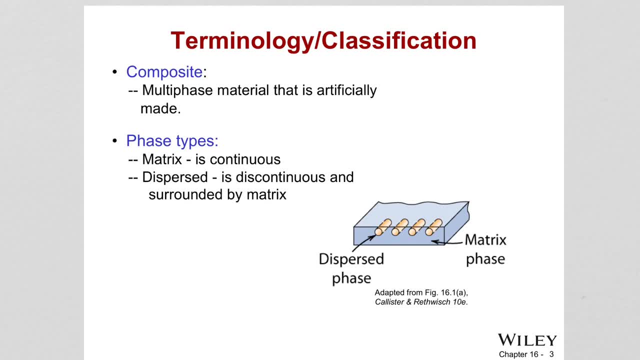 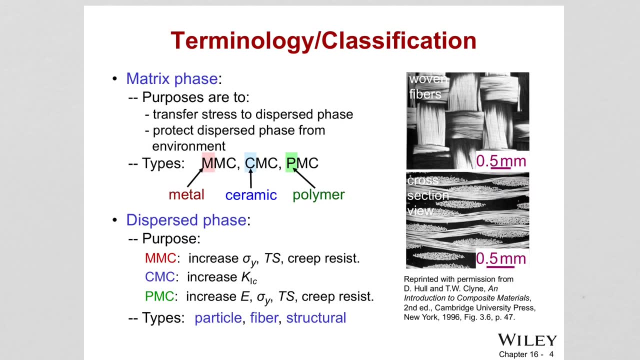 OK, so, So this is the terminology to start with. Composites might be achieved at the macro, micro or nano length scales, So you can mix two different materials phases at different length scales, Like a macro scale example is like a scale. 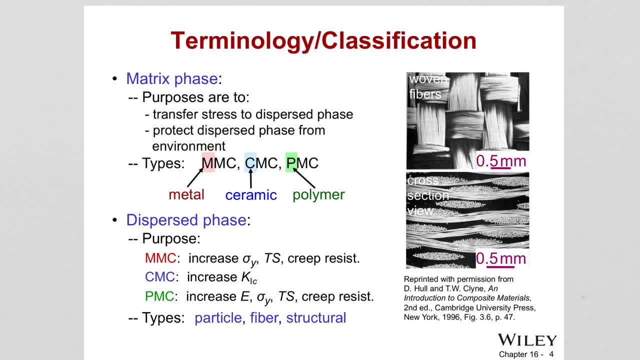 Steel reinforced concrete or micro scale is like carbon glass fiber reinforced plastics At nano scale. you can say precipitation strength in alloys like nano composites. We can give some examples to composites like space shuttle tiles consist of silica, Silica fibers and air at the same time And this exhibit low thermal conductivity. 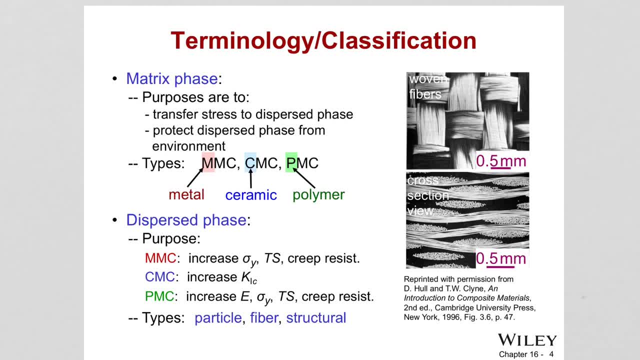 Or epoxies may be filled with silver to increase thermal conductivity, because epoxies are not conductive, thermally conductive, but silver is. So if we add silver to epoxy we are actually increasing the thermal conductivity. So we add silver to epoxy, we are actually increasing the thermal conductivity. 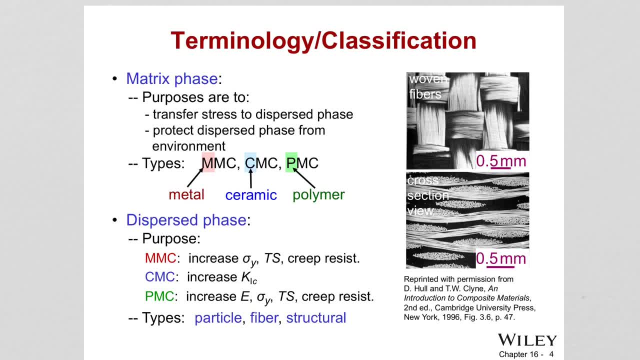 Or we can Those zirconia coating on turbine blade to provide protection against high temperatures. So making it coating on top of another material is, you can imagine it is also a composite material because we are using the properties of two different materials. So if you add silver to epoxy you will get clear, solid 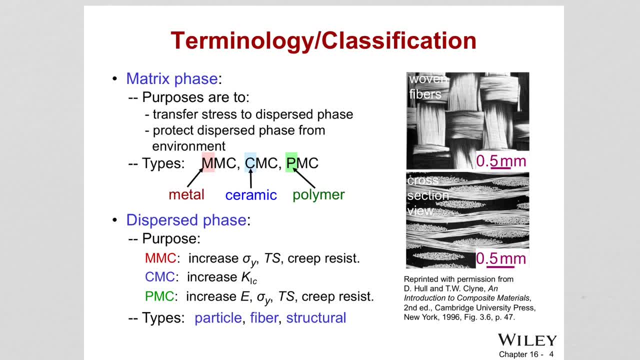 of two different materials. Now we have said there are two phases in composite matrix, which was continuous, and then dispersed phase, which was discontinuous and surrounded by the matrix. So what is the purpose of the matrix and what is the purpose of the dispersed phase? 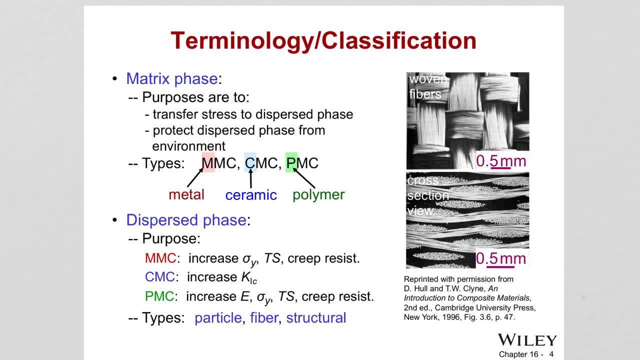 Now, the first purpose of the matrix is to transfer the stress to dispersed phase. See, we don't want the matrix to handle the stresses, because usually the matrix is not stronger, I mean, compared to the fiber, Fibers are the sources of stress. In other words, if the matrix is not 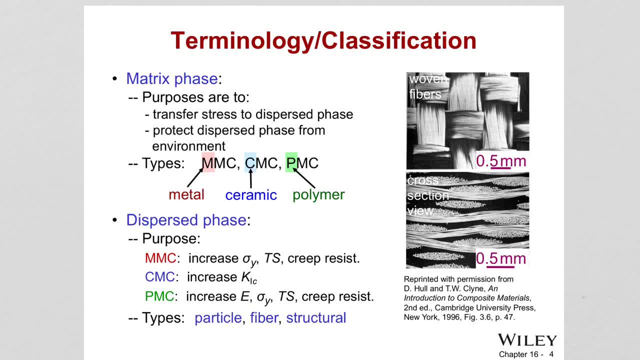 strongest phase. So that's why what you want is not the matrix handle the stresses, but you want matrix to transfer this stress to the dispersed phase, so the dispersed phase fibers, for example, then can handle these stresses because they are stronger. Another purpose of the matrix is to 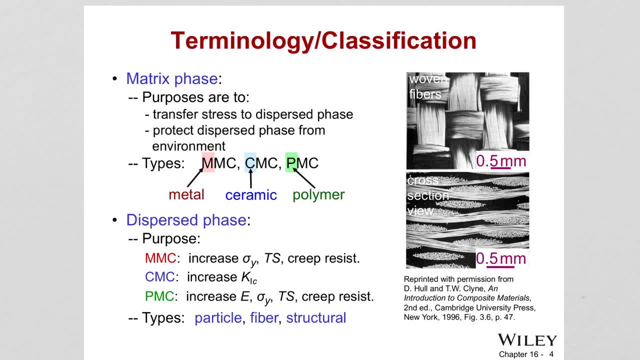 basically protect this dispersed phase from environment. So tiny particles or fibers. these are the dispersed phase and we don't want them to corrode or any type of damage to happen to them, and the matrix prevents that type of damage and protects them. So it transfers the 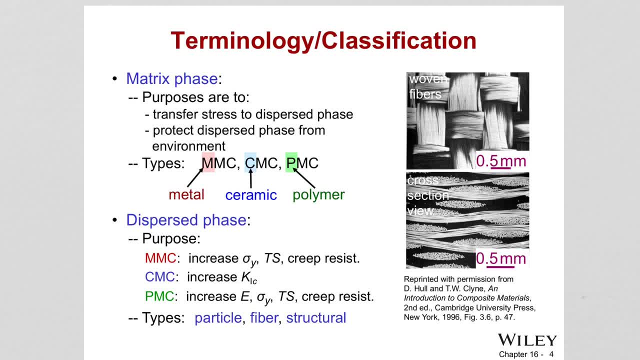 stress and it also protects the dispersed phase from the environment. It actually holds the fibers together and protect the fibers from any surface damage. There can be abrasion chemicals and it is also separating the fibers. This also prevents crack propagation that can happen from one fiber to another. 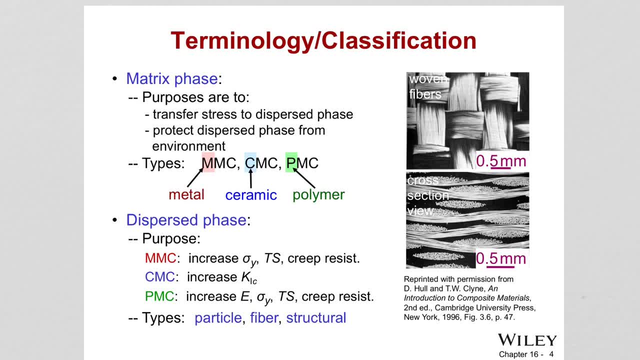 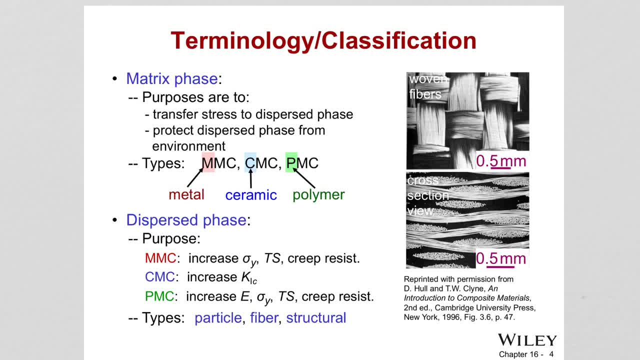 Let's see how it works. Let's see how it works. Let's see how it works. But the matrix phase determines the maximum service temperature. So there are types: MMC, CMC, PMC. Here it means it stands for metal matrix composites, ceramics matrix composites. 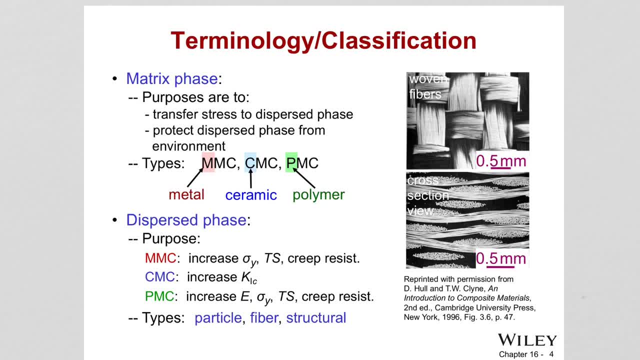 or polymer matrix composites. It depends on the type of the matrix material. Is it a metal, Your matrix material, Your matrix is a metal, ceramic or a polymer. Depending on that, the name of the composite will change. And then the dispersed phase. 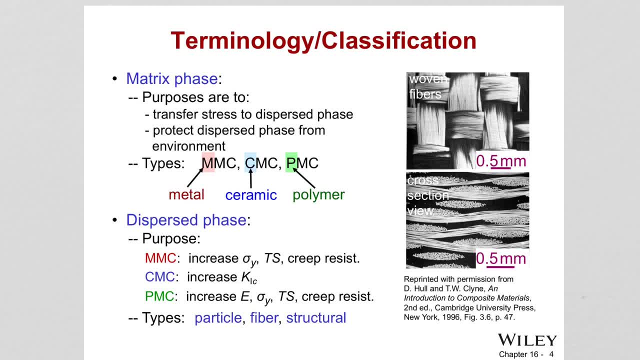 So dispersed phase can be particles, can be fibers or structural. You are seeing in the images some type of fibers are given to us, Like, for example, woven fibers. It doesn't have to be individual fibers, okay, They can be in the form of woven fibers or there. you also see the cross-section view. 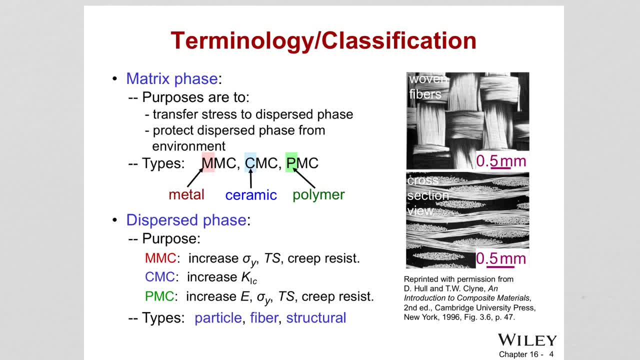 of the same thing And you can see how they are woven to each other. So they can be in any form. They can be in any form- The fiber phase, the dispersed phase- they can be not, it doesn't have to be fibers. 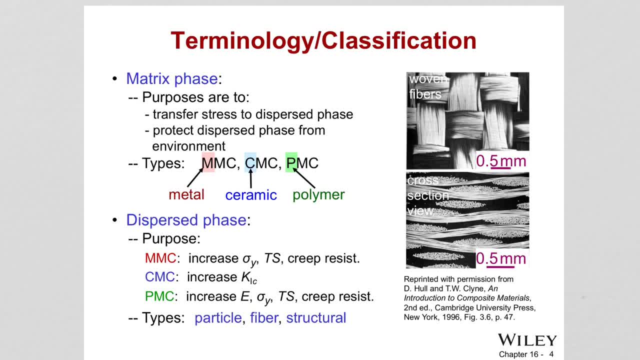 they can be particles. Fiber structural means like laminates or sandwich panels And when we say particle reinforced it can be large and particles or dispersion strengthened. And fiber reinforced can be discontinuous or continuous, So it can be in any form. There are different type of versions available. 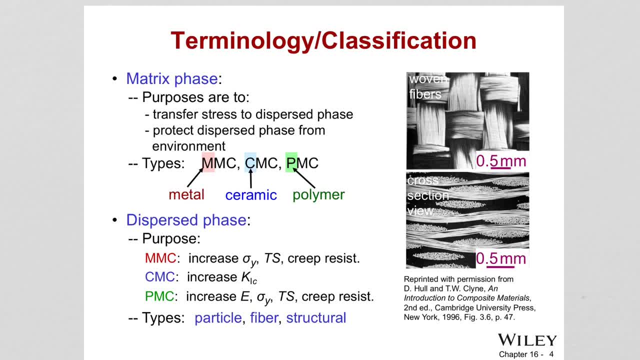 So the properties of composite will depend on the properties of these dispersed phase And then properties of the matrix phase. So it will also depend on relative amount of phases. So how much of each you have? Okay, It also depends on the geometry of the dispersed phase. 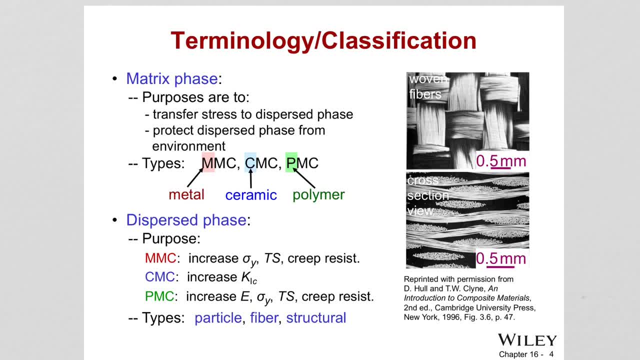 What is its size, What is its shape, What is the distribution and orientation? And it also depends on the properties, also depends on the bonding strength between the dispersed phase and the matrix, Because they need to hold each other strongly, otherwise we cannot transfer the stress from. 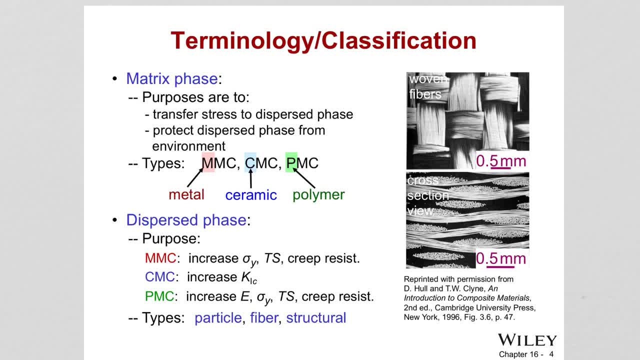 the matrix, to the fiber, to the dispersed phase. If we look at the purpose of dispersed phase in general, it will depend on what type of composite you have. When you have metal matrix composite, the dispersed phase. the idea of putting a dispersed 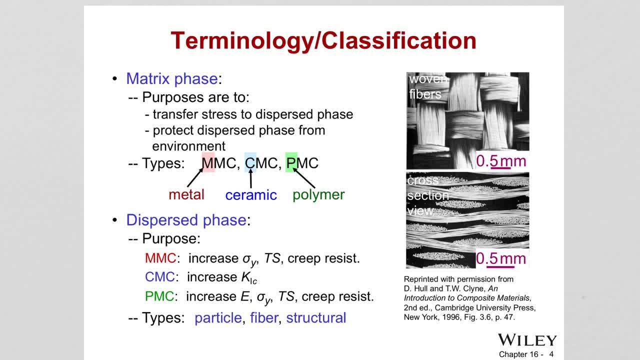 phase inside the metal matrix is to increase the yield strength, Tensile strength And creep resistance For ceramic matrix composites. matrix composites- remember ceramics are brittle, They have low fracture toughness, So the idea of making ceramics into a composite is to actually increase their fracture toughness. 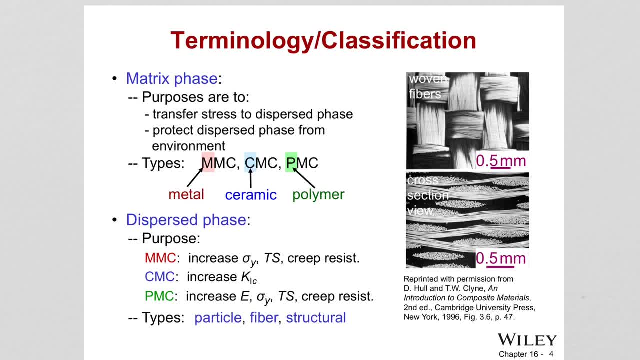 K1C. So for polymers, polymer matrix composites. you remember polymers? they have low elastic modulus, low strength, And when we actually add a dispersed phase to polymers and make polymer matrix composites, the idea here is to increase the stiffness, yield strength, tensile strength and creep. 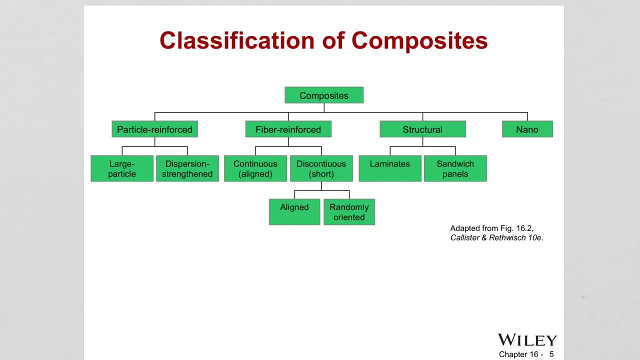 resistance. So here we are summarizing what we have learned so far. We have composites and we have different types. Like it can be particle reinforced, fiber reinforced or structural or nano. So particle reinforced is it can be large particle or dispersion strength and very tiny. 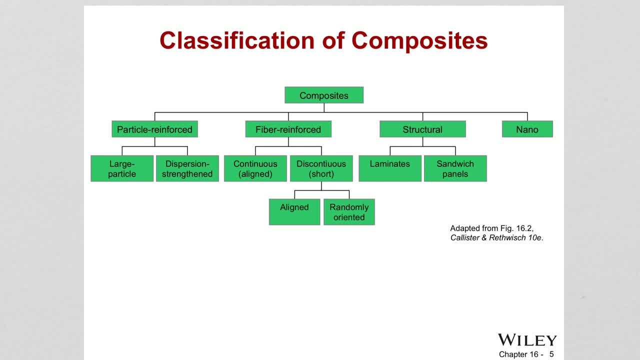 sizes like nano sizes Or fiber reinforced. These are can be continuous aligned fibers or discontinuous short fibers, and the discontinuous short fibers can be aligned Or they can be randomly oriented. So all these will affect the properties at the end. Remember the dispersed phase. this orientation and distribution affects the properties. 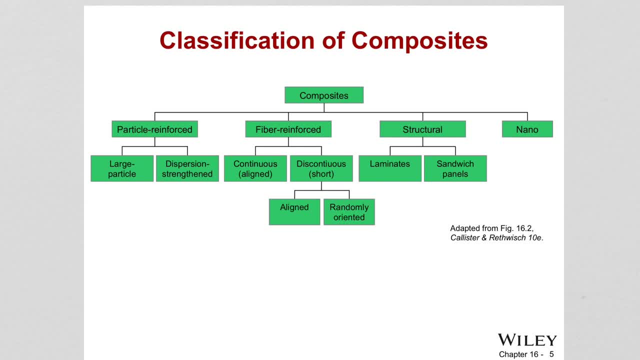 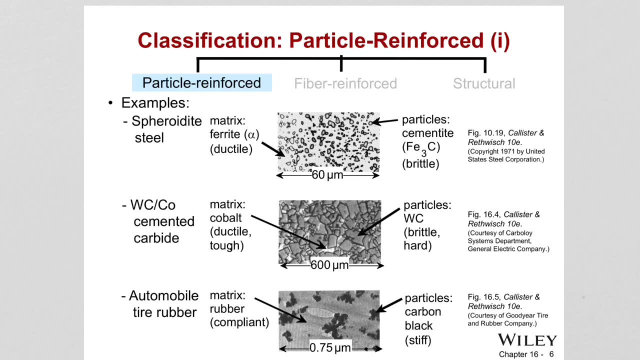 And structural laminates and sandwich panels, and there is nano composites. Now, if we take a look at particle reinforced composites, Uh, These are multifunctional. These are multi-phase materials, like pearlitic steel, Like where the alpha is soft and ductile. 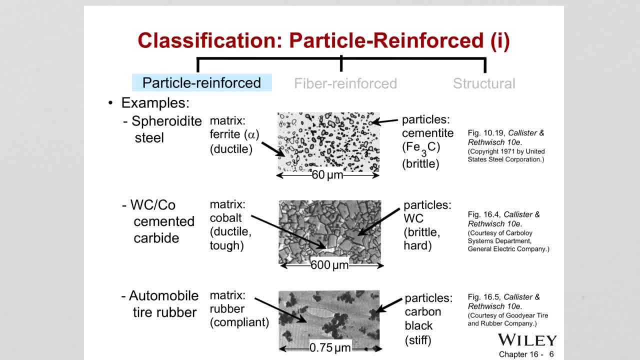 There is cementite which is hard and brittle And pearlite makes a high ductility and strength due to the presence of both cementite- as hard and brittle cementite and soft and ductile ferrite, So similar to that. we have examples, For example sepharodite steel. 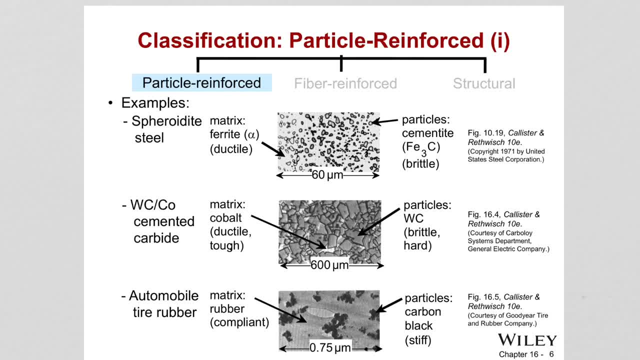 The alpha matrix is ferrite, Ductile ferrite. The alpha matrix is ferrite, Ductile ferrite, And there is cementite particles. that is brittle Again. this provides ductility and hardness at the same time. So strength and ductility at the same time, as you can see. 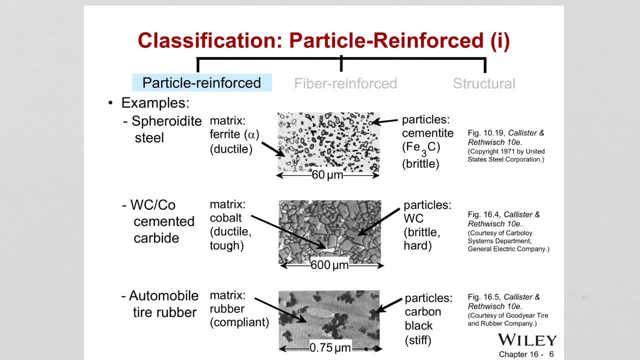 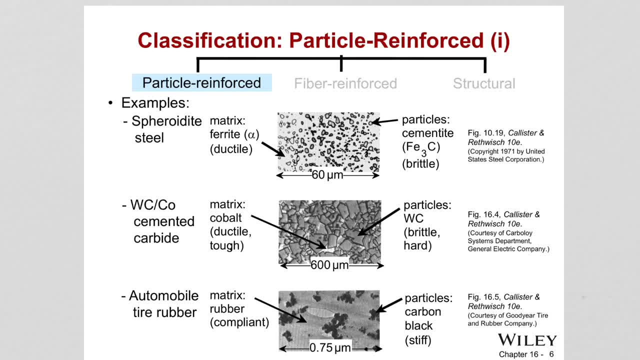 And you guys are also seeing the microscopic images. They are identifying which ones are the particles, which is the matrix itself. So in this case, the matrix is cobalt, which is ductile and tough, But the tungsten carbide is a ceramic. 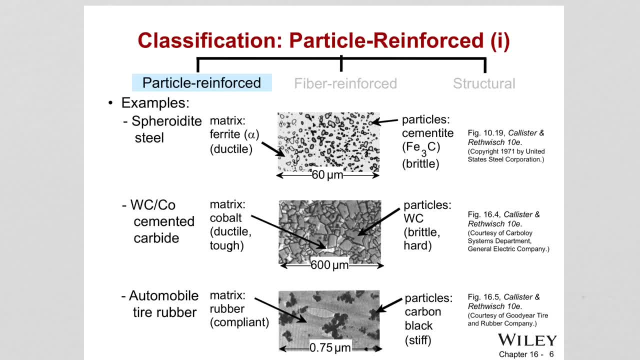 We know it is hard and brittle, so you achieve strength and ductility at the same time. and there is another example: automobile tire rubber. the matrix is rubber and the particles are carbon black. so remember, rubber is actually whitish, right. so you have you ever questioned that? why actually car tires, even if they are made up of rubber? 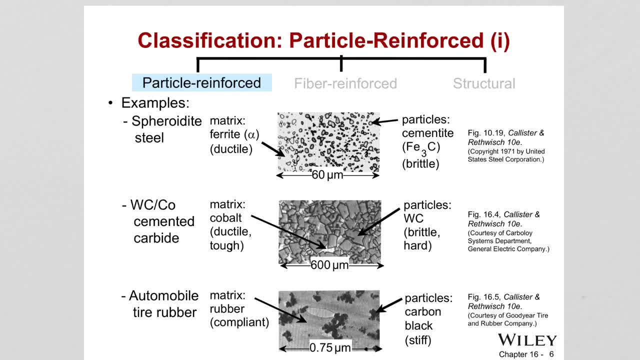 why they are black. so, the fact is, the reason they are black is because there is carbon. black is added as a reinforcing filler in rubber products, especially tires. so there are some fillers added to the polymeric materials, and an example of this is carbon black as an 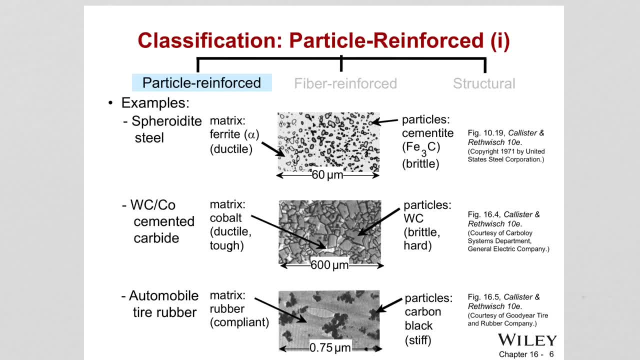 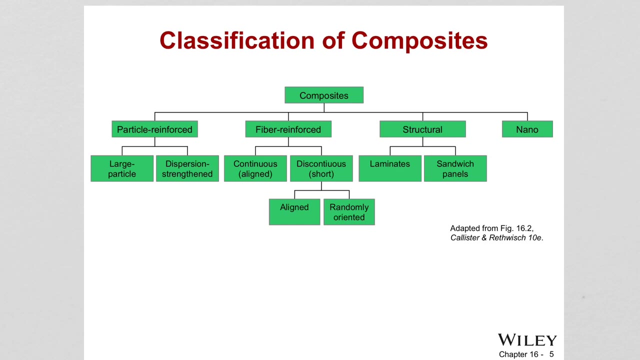 example of carbon black being added to a car tire, isn't it? and needing to be to the rubber. so this is done in order to improve tensile and compressive strength, toughness and thermal stability of polymers, in this case rubber. in particle reinforced. large particle reinforced, or what was it? dispersion strengthening. so in 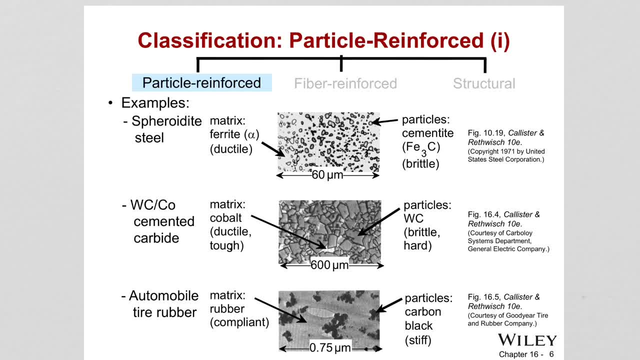 particle reinforced polymers, the particulate phase usually harder and stiffer and particles restrain the movement of the matrix phase in the vicinity of each particle. matrix transfers applied stress to the particle, so the degree of improvement of properties will depend on the bonding strength at the matrix and particle. 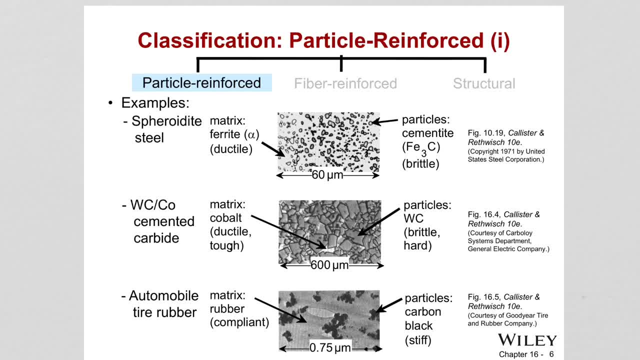 interface. the idea here is particles approximately the same dimensions in all directions will give you a uniform achievement of enhancement in properties. they should be small and evenly distributed for effective reinforcement. another example to this can be given for aluminum alloys for automotive connecting rods and pistons. they are being strengthened. 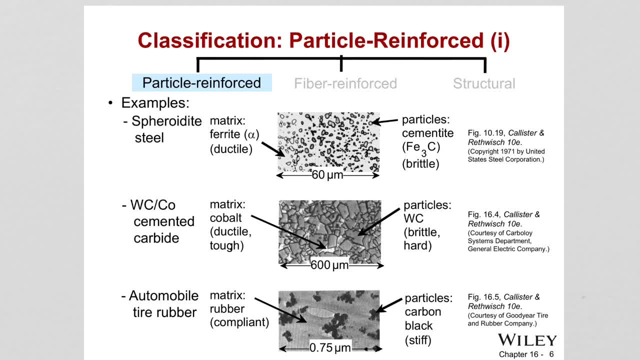 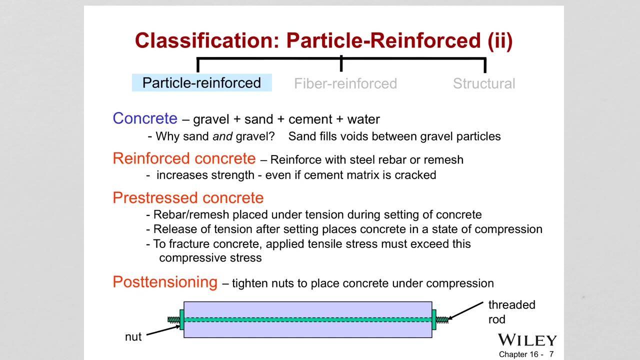 and hardened by addition of silicon carbide particles, silicon carbide being the hard phase, stiffer phase, which is added to the aluminum to to basically strengthen the material. so we can use them in connecting rods and pistons. other example is concrete, which is a composed of cement, the matrix. 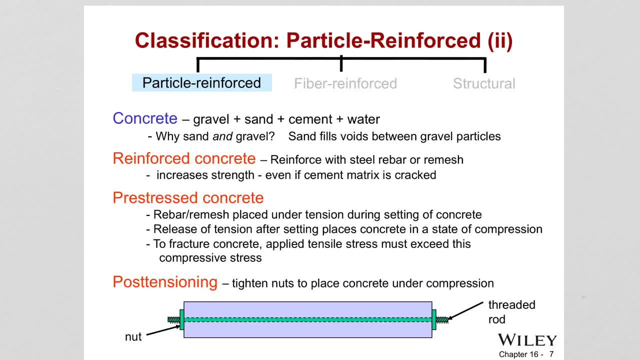 and sand and gray oil particles. so matrix and dispersed phases are ceramic here and there is reinforced concrete. the strength of the concrete may be increased by additional uh reinforcement. this is usually accomplished by means of steel rods, wires, bars or mesh which are embedded into the fresh and uncured concrete. so the reinforcement then gives the hardened 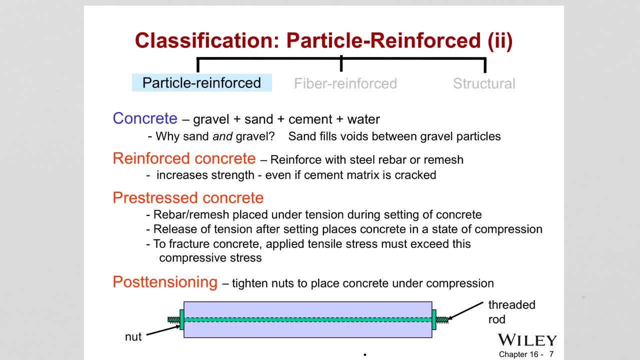 structure to support greater tensile, compressive and shear stresses. even if there is a crack, it can develop. in concrete we know ceramic material concrete, so even if it can develop- i mean the composite but made up of ceramic materials here- if there is a crack develops. considerable reinforcement is maintained when we reinforce the concrete with steel bars. 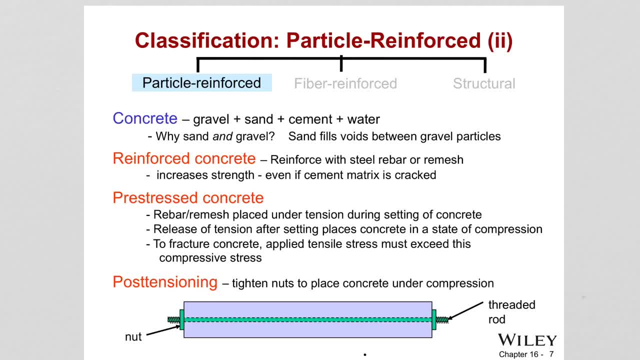 another reinforcement technique is the concrete. reinforcement technique for strengthening concrete involves the introduction of residual compressive stresses into the structural member. this, this is called press stress concrete and remember the materials are not good in tension right ceramic materials. so if you actually put compressive stresses initially, if you press stress the concrete, it will count. countering: 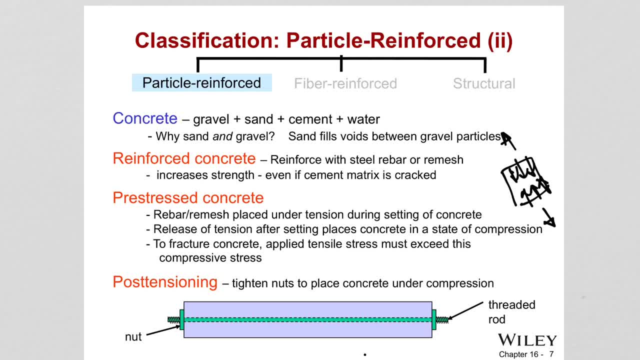 to interact with the tension. so this way you increase the tensile strength of the ceramics. so this method is used for brittle ceramics. they are stronger in compression than in tension. and then for this fracture of this stressed concrete member to happen, the magnitude of the pre-compressive stress must be exceeded by an applied tensile stress. so that is the whole idea. 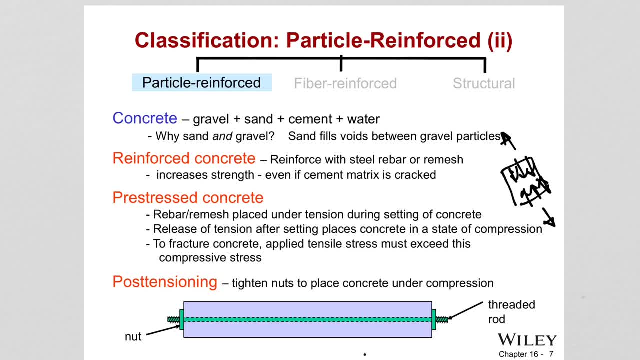 post tensioning is another way to form reinforced concrete here. actually, you can understand this. think about: you have a rubber band and a series of wooden blocks with holes drilled through them and and into which a rubber band is threaded, and if you hold the ends of the rubber band, the blocks, 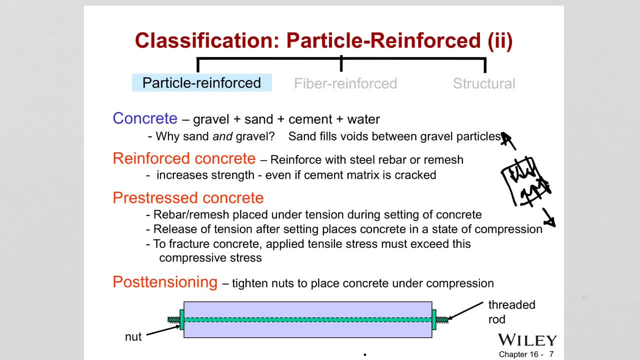 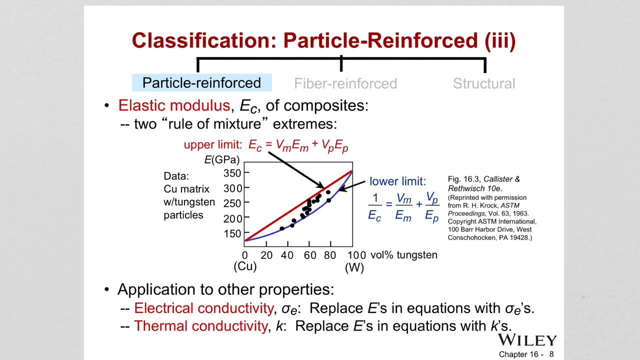 will sag, but if you actually tighten the rubber band right and the blocks will remain straight. so this is the idea behind this: so tightening the steel rod, so tightening the steel rod and so that it will hold the concrete in place under compression. now let's look at the dependence of elastic modulus on the volume fraction of the constituent phases. 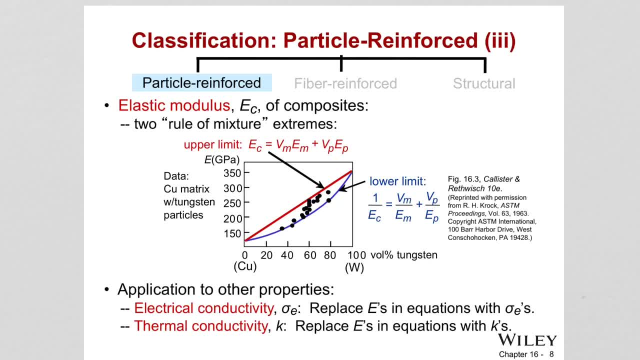 now let's look at the dependence of elastic modulus on the volume fraction of the constituent phases for a two phase composites. so here there is a rule of mixture. this rule of mixture accurately provides a theoretical upper and lower bound on the properties such as elastic modulus density, ultimate tensile strength. 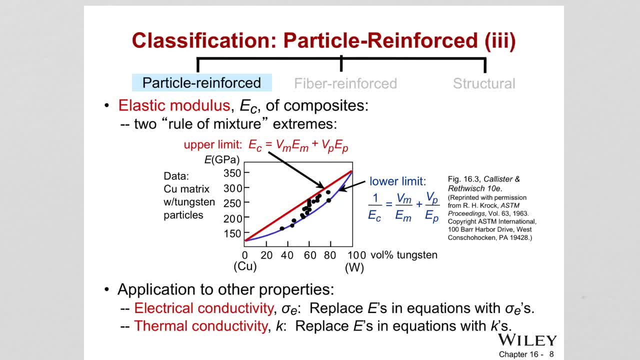 thermal conductivity and electrical conductivity. so remember, we are mixing two different mixtures and doing some research. we have found that mixedmatte environments of his is affected by electrical conductivity. butและство 풀 rant 1930 aliexer aるبین��ographicнőne. 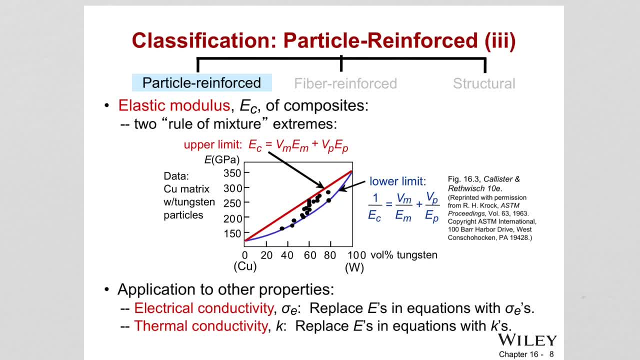 we apply two phase components. we do not require a dual phase compound. so from here, as a combination-basic understanding, we use four phase components, different materials, and the question is: how are you gonna calculate its modulus, or how are you gonna calculate its density, how are you gonna calculate its tensile strength, or how are you? 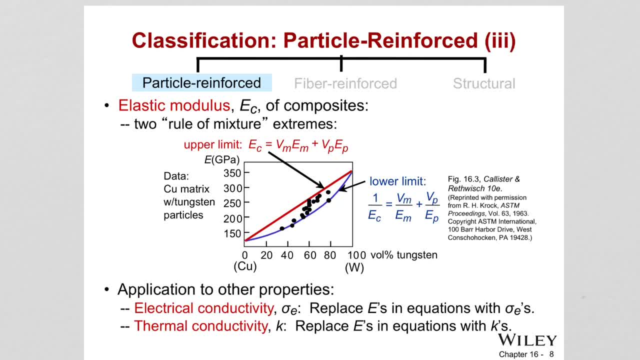 gonna calculate its thermal conductivity. usually the best way is to do experiment and get the result. but those experiments or the data which you're seeing here as the black dots, which is collected from experiment- okay, those experimental data, for in this case the y-axis is modulus and the x-axis is percentage of tungsten added to copper. you see the actual data, experimental. 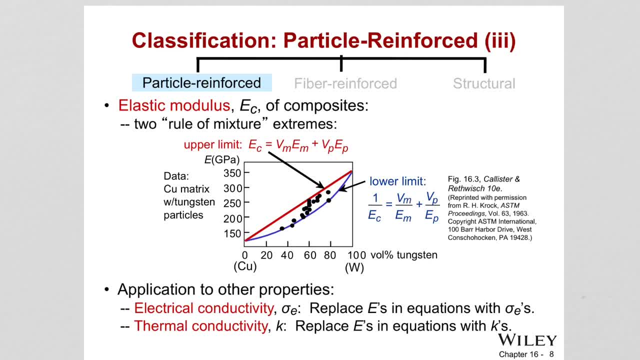 data is in between limits, limits, lower limit and upper limit, and upper limit is shown with the uh red and lower limit is shown with the blue. this upper and lower limit. these are calculated theoretically with an equation and rule of mixture equation. it provides us the upper bound and lower. 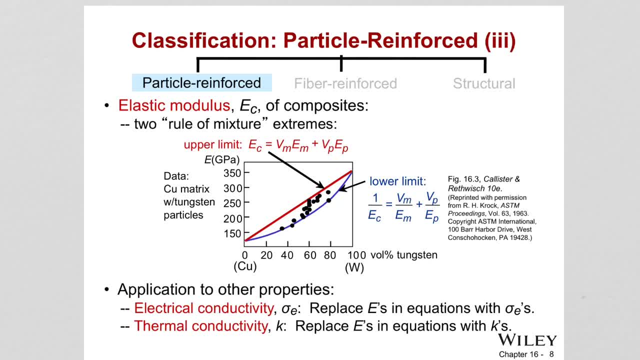 bound that we should expect by mixing those materials. it doesn't give us the exact. the exact solution can only be done with the experimentation and collecting data points, like we are seeing in the black dots. anyhow, those black dots needs to be located somewhere in between these limits. 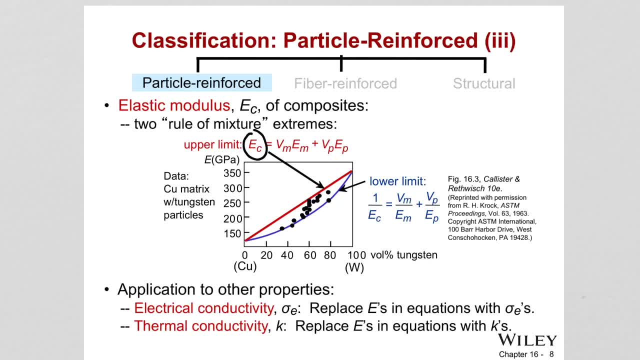 in this case the modulus of the composite shown with ec. they will depend on, in the upper bound, the volume fractions of the each constituent. so volume fraction of the matrix, times modulist of the matrix, plus volume fraction of the particle, times elastic modulus of the particle. this equation forms the upper limit shown with the red. the lower limit is true. this equation. 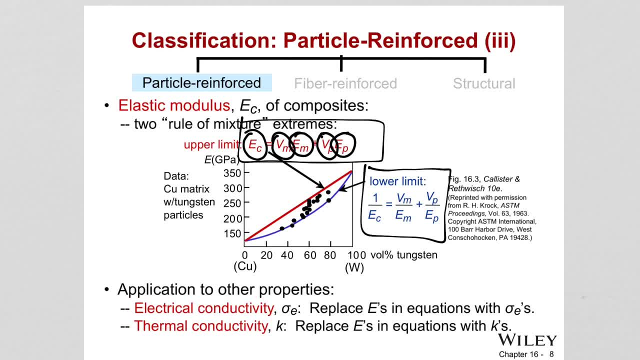 okay. so 1 over ec, which is the composite uh modulus, is volume fraction of the matrix over the modulus of the matrix, plus volume fraction of the particle over the modulus of the particle. so this is to find the lower limit. I will not go into derivations of these equations. there are: 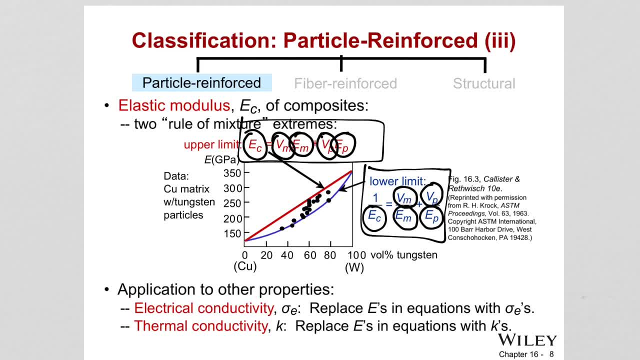 reasons why these equations are derived this way. you, if you're interested guys, you can look for it online and you can see how they actually derived it, but it is in not in the scope of this class. okay, just like the modulus, you can apply this technique to any other property, like electrical conductivity or. 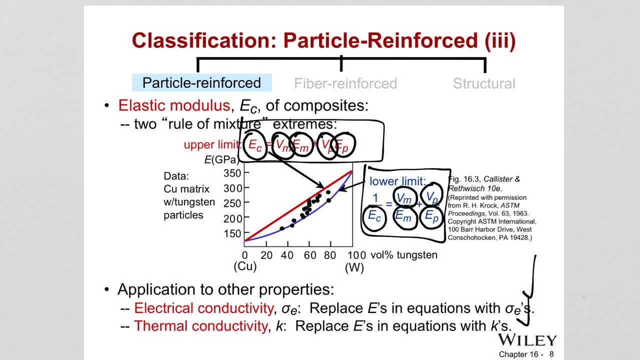 thermal conductivity. so instead of the modulus you replace them with the electrical conductivity. and instead of modulus you can replace the equations with K, which is the thermal conductivity. at the end, idea is the same. those are theoretical limits, extremes, max and means that the data points can have, but actual results are from. 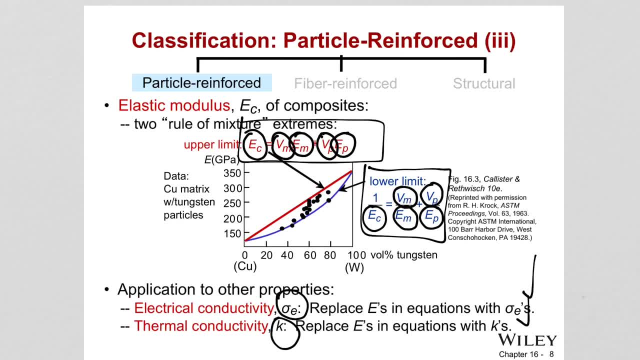 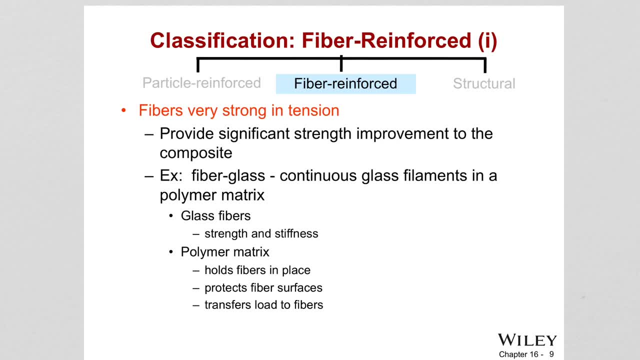 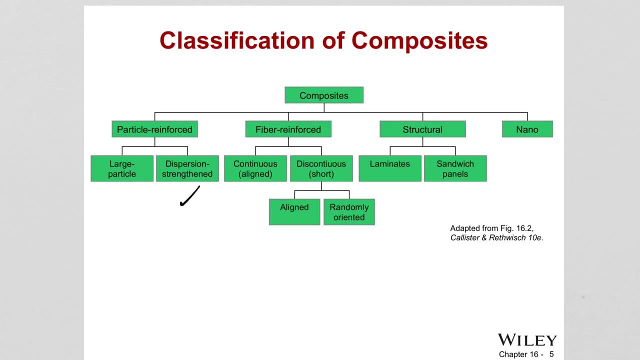 experiments. you collect data from experiments here before going into fibers, a fiber reinforced void, reinforced composites- remember we also have these person strengthen here. what does that mean? that means we have particles that are very small, like oxides. in a structure like this, particle size is tall. 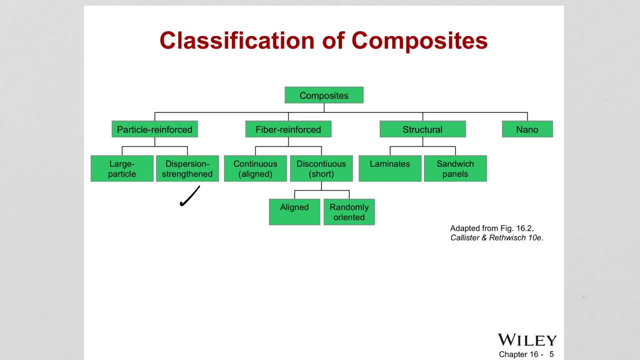 to 100 nanometer. Strengthening in this case occur at atomic or molecular level. And strengthening mechanism in dispersion strengthen materials is similar to precipitation hardening, which will impede the dislocation motion. Since the dislocation motion is impeded, that the plastic deformation is restricted. therefore the yield strength and tensile strength. 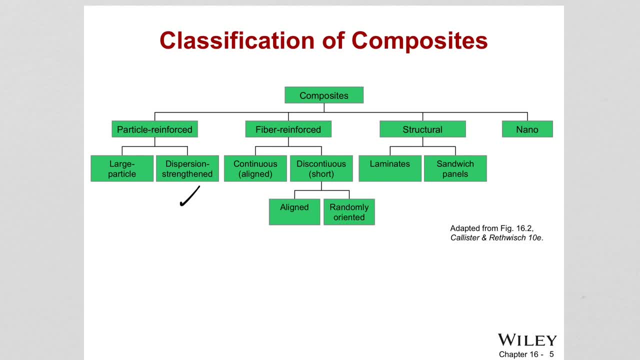 and hardness improve. The good thing, actually, for dispersion strengthening is, unlike precipitation hardening we employed for aluminum alloys, strengthening can be retained at elevated temperatures Because, remember, in precipitation hardening we are using the alloying system to form precipitation, But in this case we are intentionally dispersing tiny particles ourselves which will retain their. 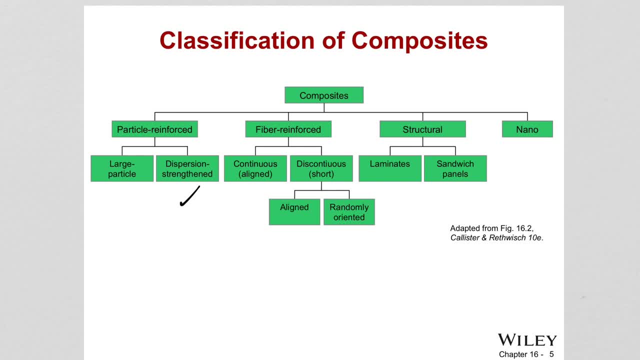 strength at elevated temperatures. One example to this is theorea dispersed metals: Theorea dispersed metals Like TD, TD, chrome, TD, nickel. These are high temperature structural materials that are being used in like gas turbine engines, And in your book it should, there should be an image and there should. 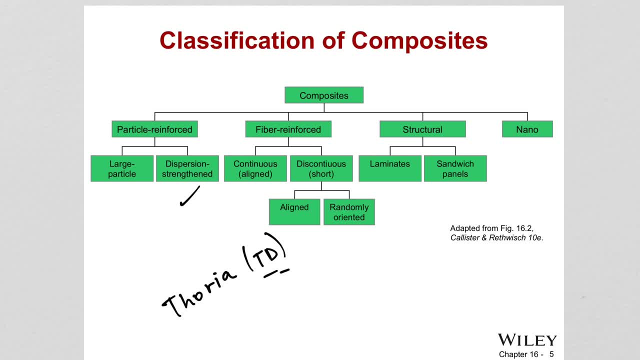 be also a table if you're interested to see applications of different dispersion strengthen composites. Some examples in my mind is like silver mixed with cadmium oxide, used for electrical contact materials. Aluminum mixed with alumina, possible use in nuclear reactors. Beryllium mixed with. 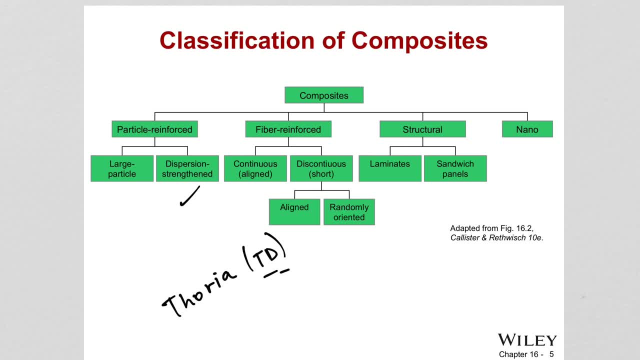 beryllium oxide particles. These are aerospace and nuclear applications, nuclear reactor applications, etc. So the idea here is tiny, small oxide, This strong particles, being dispersed in the metal matrix here. okay, that's the whole idea, similar to the precipitation hardening, but in this case you manually add these. you are not. 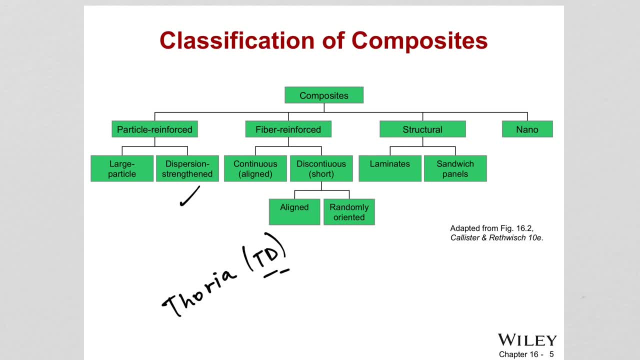 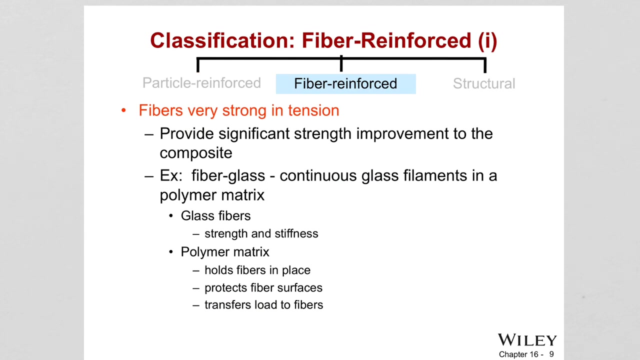 using the alloying system itself to form the precipitates. you are manually adding, intentionally adding those particles to achieve strengthening and therefore it retains its strength at elevated temperatures. so now we can go to fiber reinforced palm composites. i'm sorry so fibers, fiber reinforced fibers. they are very strong in tension. 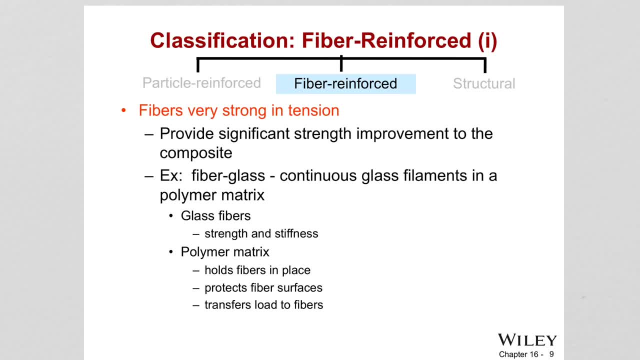 therefore, they provide strength to the composite. one example is fiberglass, continuous glass filament in a polymer matrix composite, so we call this fiberglass or glass fiber, polymer matrix composite materials. in this case, the glass fiber is the discontinuous phase, which is strong and stiff, and the matrix is polymer. what it does is holds the fiber in place. 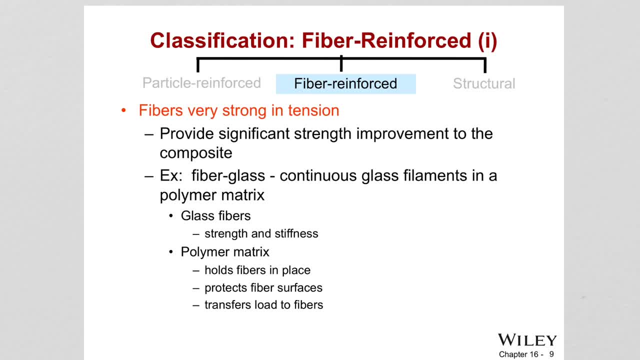 as we talked about, and protects the fiber surfaces. if the fiber is loose or lose, it will bring the stresses up and it will transfer through the matrix and in the matrix you will be able to see that the fiber is transferred to the fiber. but if the fiber is low, it will transfer its load to the fibers because the fibers are the stronger. 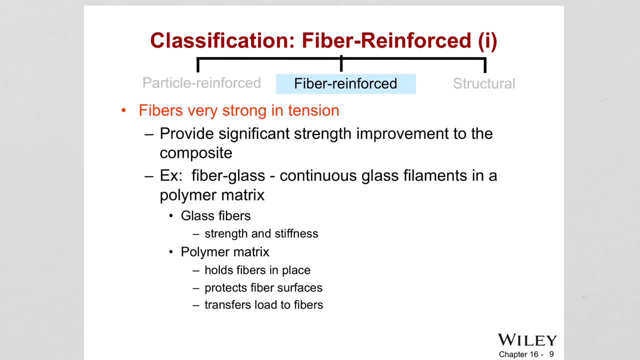 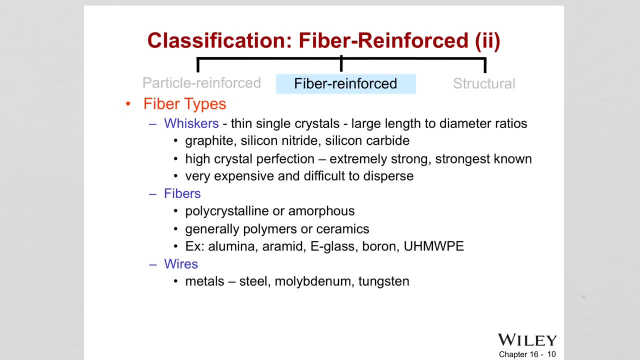 phase. they will carry the stresses instead of the matrix. that's the whole point here. make the matrix transfer the load to the fibers so that it can handle the stresses phase. First of all, think about the small diameter of a material is much stronger than the bulk form. 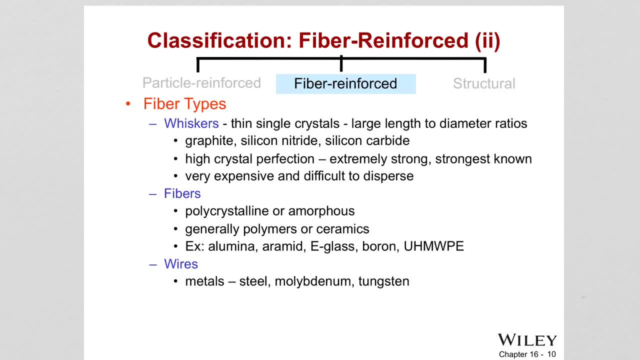 So if you make any material in the fiber form, it will be stronger than its bulk form. The reason is the possibility of finding defects is decreasing. They are becoming like nearly defect free. So remember, defects are the reasons where there is stress concentrations and therefore 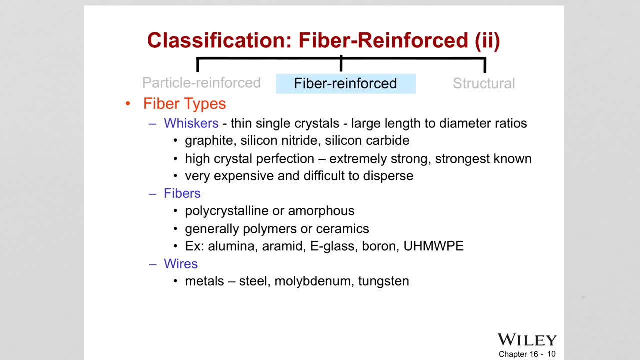 failure of material happens. Therefore, as we make the sizes smaller, the possibility of finding defects in the structure is lowering down, and this is strengthening the materials compared to their bulk form. So any type of fiber can be created from any type of material, but they will be stronger than their bulk form, And the types here are whiskers, fibers and wires. 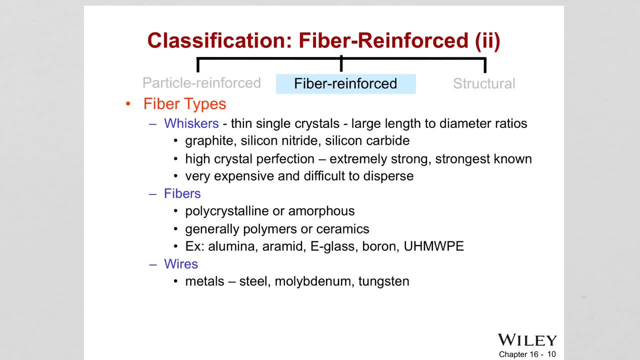 So whiskers are very thin single crystals that have large aspect ratios. Aspect ratio means length over diameter And among the strongest known materials due to no mobile dislocations. the whiskers are, And examples are graphite, silicon, carbide, silicon, nitride, aluminum. 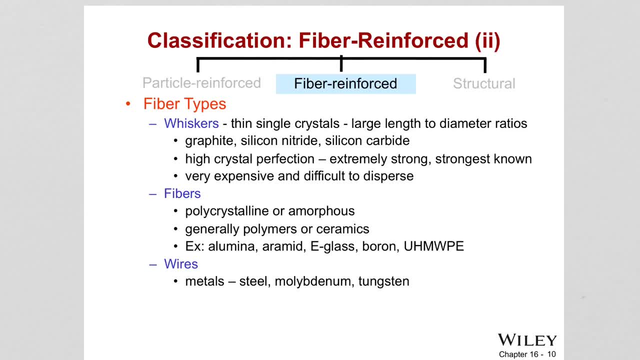 oxide. They are all possible in whiskers form Also, fibers. Fibers are like polycryst, can be polycrystalline or can be amorphous, And these can be generally polymers or ceramics like alumina, aramid fiber like kevlar, e-glass. Different type of glass fibers are available. One of them is e-glass. 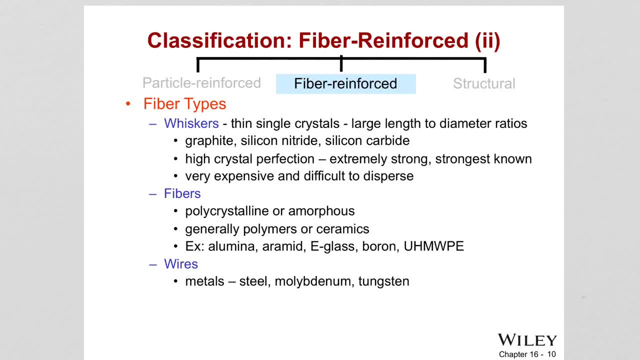 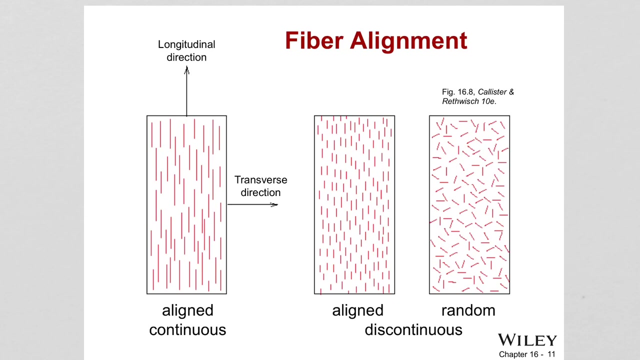 and boron and ultra high molecular weight polyethylene. And the wires. The wires are like relatively large diameters, like steel wires or molybdenum wires or tungsten wires. So again the idea here: in fiber reinforced composites we have strong, stiff but brittle fibers. 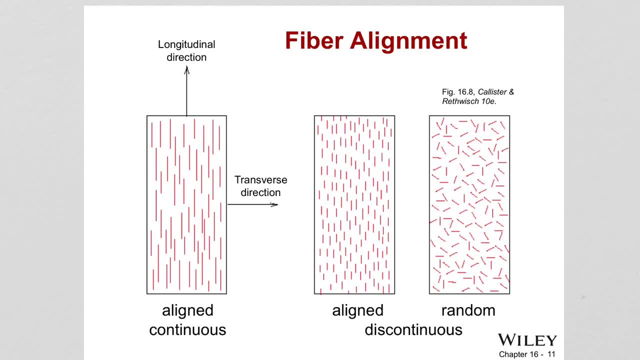 in a ductile. So we can say that this is a very strong matrix. It improves the strength and modulus and fatigue resistance And the key here is, of course, when we reinforce the matrix, the composite itself will have a modulus that is higher than those of their matrices And properties like modulus of composites. 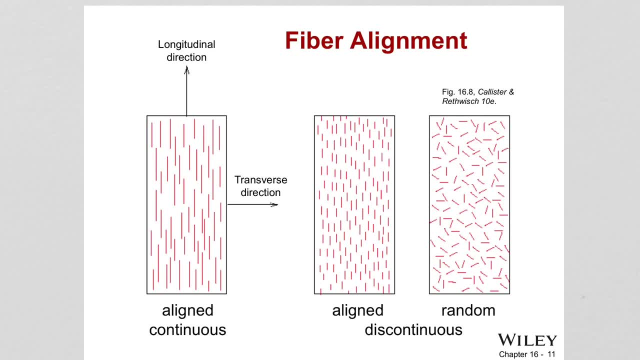 can be very anisotropic, Meaning that the modulus is higher in some directions than the others. This is sometimes desired. They intentionally increase the modulus in certain directions, Like when you are using composites to build vaulting pole to achieve stiffness only on. 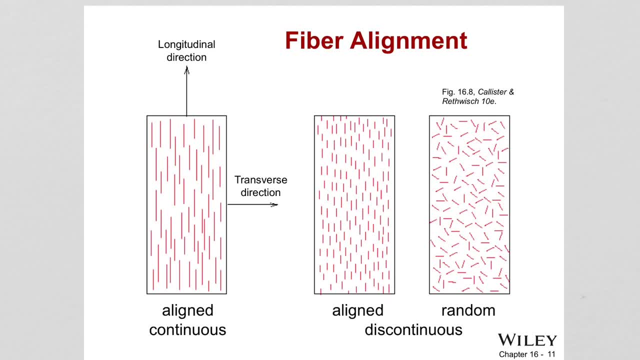 certain bending direction or rackets, etc. This is intentionally can be done. So what do we mean? the properties Depends on the direction, Like: why is it anisotropic? And it is because of the fiber alignment in the structure through the matrix. 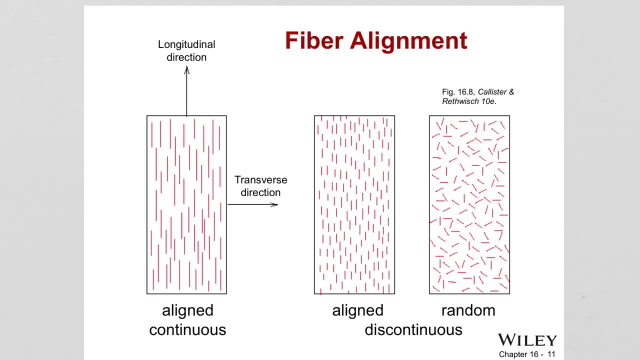 First of all, continuous fibers can be aligned and continuous, like this one, And there are discontinuous fibers that are aligned, Like this one, Which are shorter and aligned, And there are discontinuous and random, distributed fibers, Like this one. All of them will have different properties. 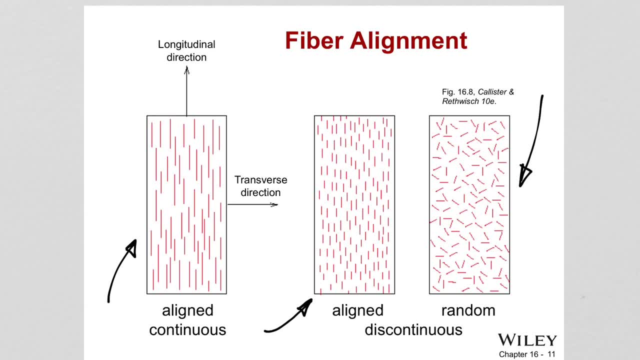 But better overall properties are realized when the fiber distribution is uniform. So, as I said, the properties of a composite having its fibers aligned are highly anisotropic and depend on the direction which they are measured. If you see, the enhancement in properties in this case will be achieved in longitudinal direction. 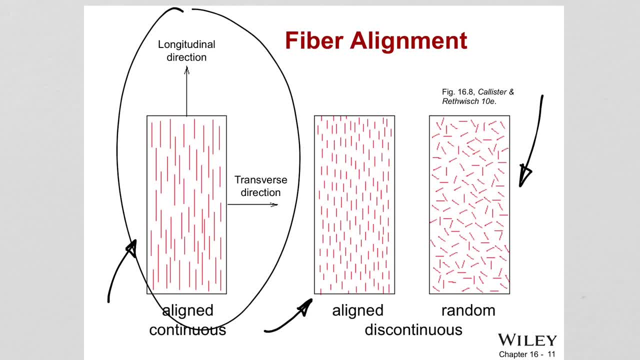 But in transverse direction, you won't observe any significant enhancement in the properties. So in this case, and in this case, As you see, the fibers are aligned. Therefore, the properties will depend on the direction and it's going to be anisotropic. 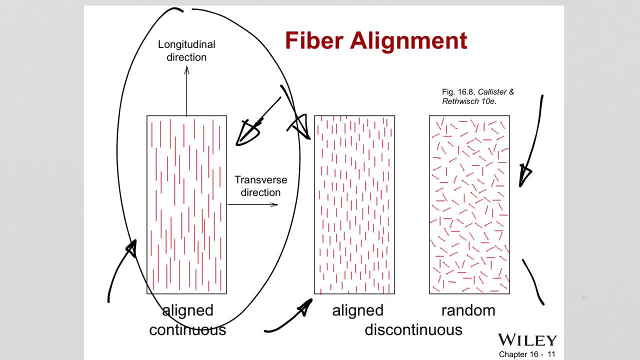 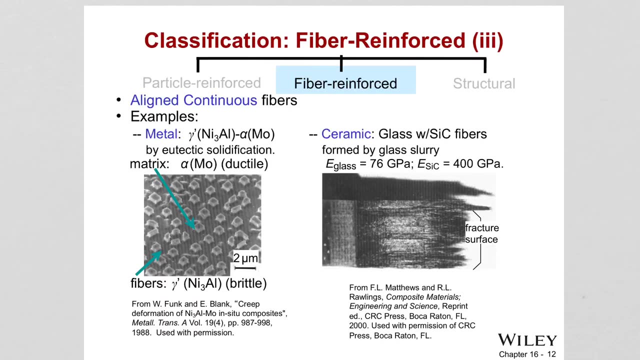 However, if you have random distribution, just like this one, Then you achieve enhancement in all directions. So, as you see how the fiber orientation can influence the properties, All right, so we have examples here We are seeing an example if the matrix is metal or if the matrix is ceramic. 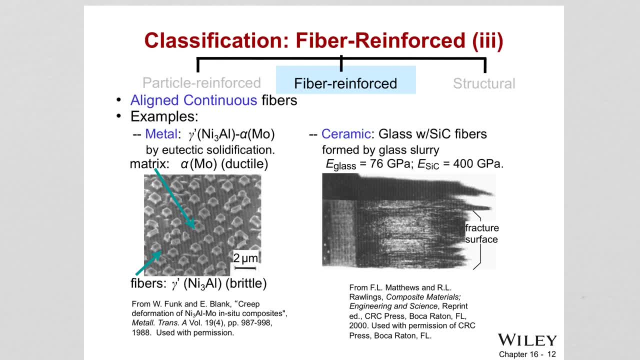 What are some examples to this? It is nickel aluminide in molybdenum matrix. As you see, molybdenum is the ductile phase, the metal, And nickel aluminide is the basically the ceramic brittle phase, And we are seeing a microsquare. 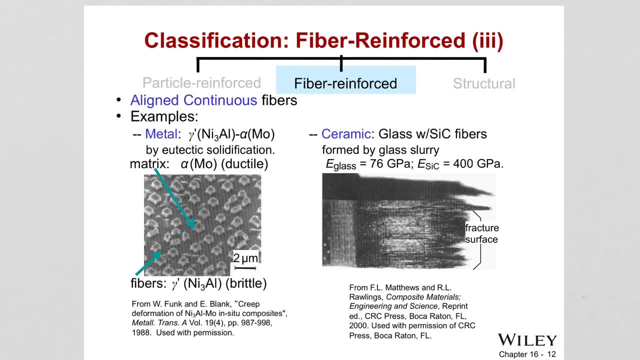 And we are seeing a microscopic image of the fibers that are getting out of the matrix phase. We are seeing that it must be an image from the edge of the sample. So here in the ceramic matrix which is reinforced with silicon carbide fibers, As you see, some image is given here. the silicon carbide has a better modulus than the glass. 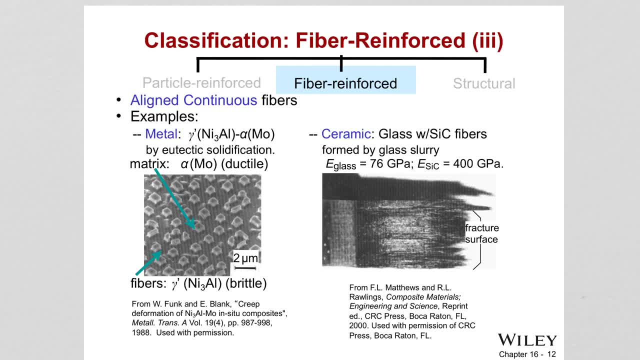 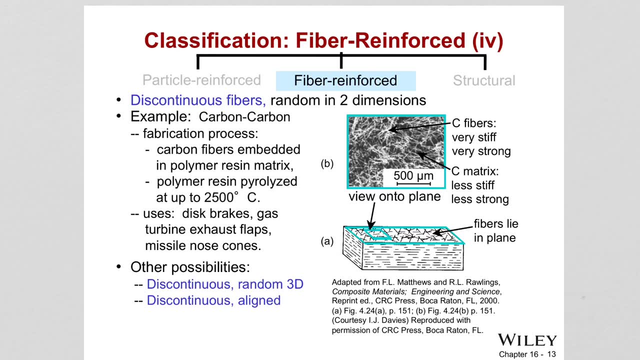 So it is to enhance the modulus of the glass phase. basically, We continue with examples how this continuous fibers- That means they are randomly, and random in two dimensions, Meaning randomly distributed- It can be also aligned, okay. So we have seen that. So here we are, seeing that. 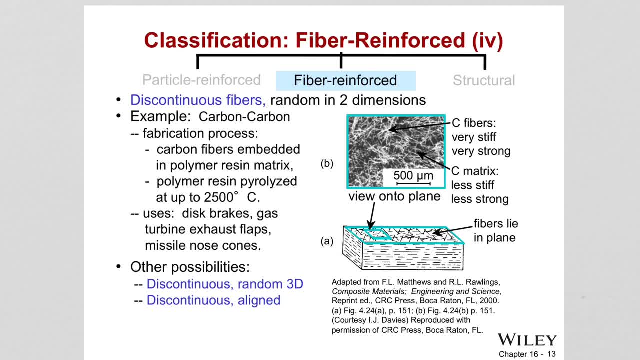 Here in example, is given to us carbon, carbon fiber, reinforced composites. All right, the image is here: carbon fibers We are seeing very stiff and strong within the carbon matrix, Which is less stiff and strong. Remember, the carbon can have different structures, right? 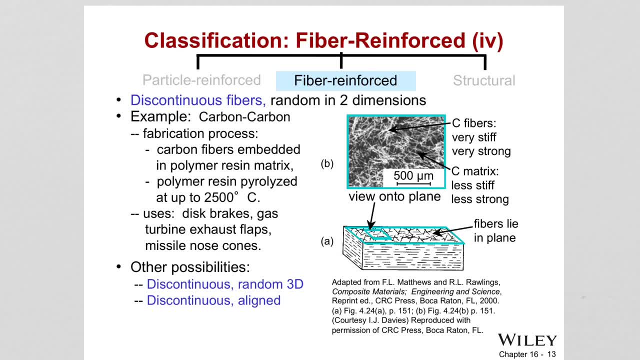 So and the fiber form will always be stronger In the matrix itself. So here how it is done: Carbon fibers Fiber is embedded in the polymer resin matrix And this polymer is pyrolyzed, Meaning it turned into carbon. So at high temperatures it decomposed and formed carbon inside the structure. 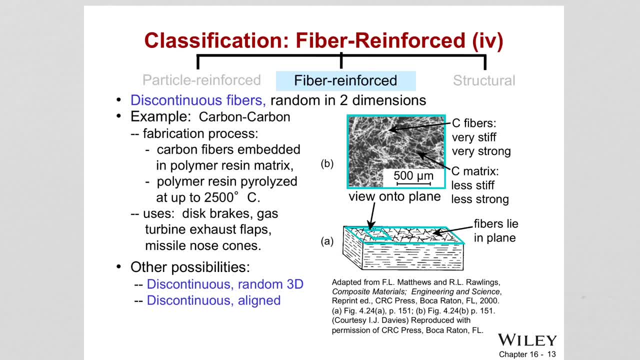 So this forms how. this shows you how the carbon carbon composites can be done, And I also suggest you guys watch the videos I sent you If you're interested- how the carbon fibers are formed etc. And use of carbon carbon composites in f1 formula cars- f1 cars. 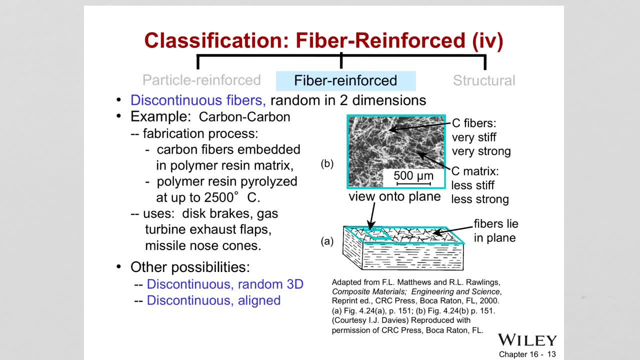 So you can watch those videos. But this type of structure, I should say It is very, very strong and very expensive type of composite, Carbon, carbon composite- And they can retain their elasticity and last high modulus of elasticity and tensile strength Up to 2000 degrees c's. 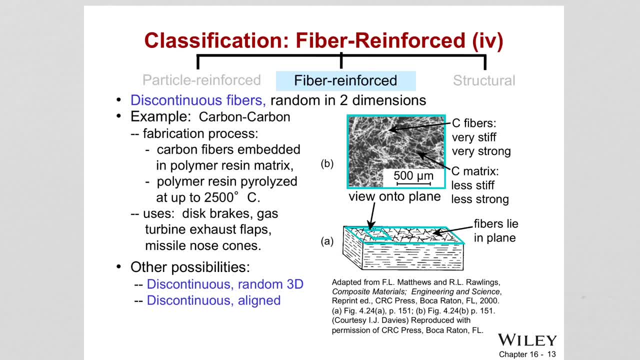 Very good: creep resistance, High fracture toughness, Low thermal expansion, High thermal conductivity, High thermal shock resistance. So these carbon carbon composites are used in space: shuttle nose, tip and leading edges, Rocket nozzles and tips, Air ducts, Aircraft. 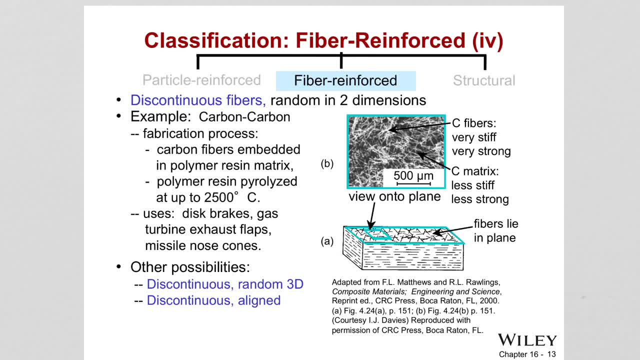 F1 racing cars and train brakes. So this is a very expensive material And we are seeing here how it is made And those fibers can be aligned or they can be random in 3d. And if they are aligned, remember it's going to be an isotropic. 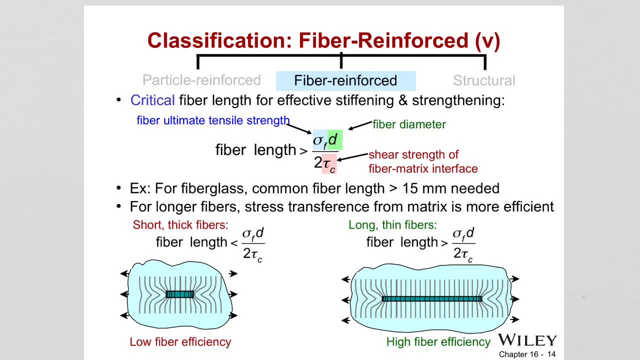 Okay, so there is the influence of the fiber length, So there has to be a critical fiber length necessary for effective strengthening and stiffening to happen. Remember, the fibers needs to carry the stresses And if you want to effectively the matrix, to transfer stresses to the fiber. 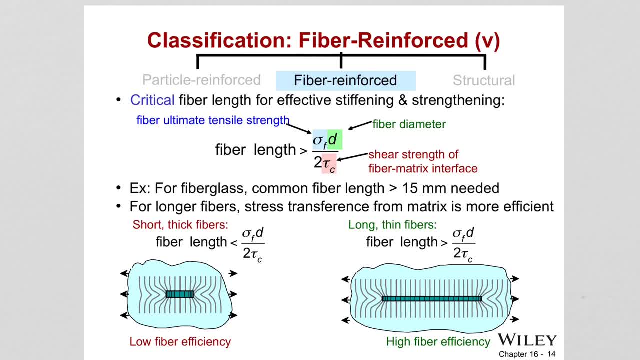 The fiber has to be at a certain length, Otherwise you cannot achieve effective strengthening or stiffening, And critical fiber length Depends on the tensile strength of the fiber and then fiber diameter and the shear strength of the fiber matrix interface. That's the reason why we said that the bonding between the fiber and the matrix should be strong in order to achieve good transfer of the stresses. 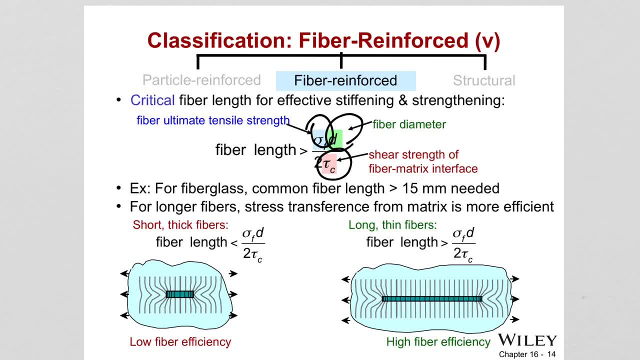 In order to achieve effective strengthening, In order to achieve effective strengthening, In order to achieve effective strengthening. Okay, so this fiber length will, of course, given the it depends on the tensile strength and interface strength, etc. It will change from different fibers to different fibers. 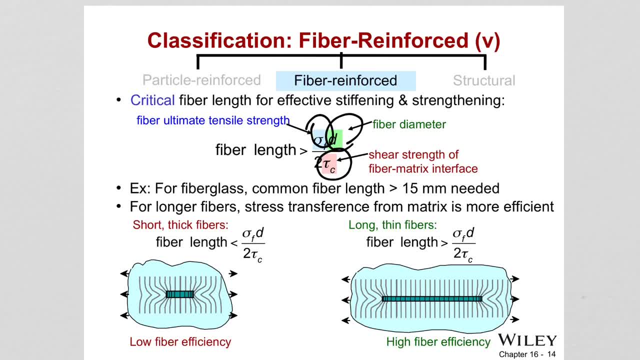 For example, for fiberglass, common fiber length is above 15 millimeter to achieve this effective strengthening. So for long fibers, stress transfer from matrix matrix is more efficient As we go above and if, if, as we reach and go above the critical, the critical fiber length. 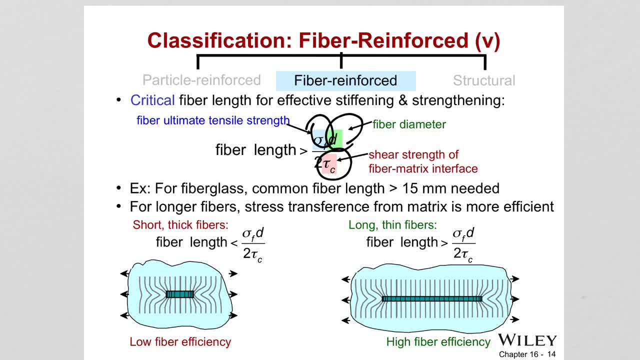 We are achieving better strengthening, more efficient strengthening. okay, So the idea here is: let's say, the capacity of long fibers is greater than larger fibers, Transforming it to build. listened, the fiber is to carry 6 gigapascal. let's say I'm making up, okay, so you want this whole stress? 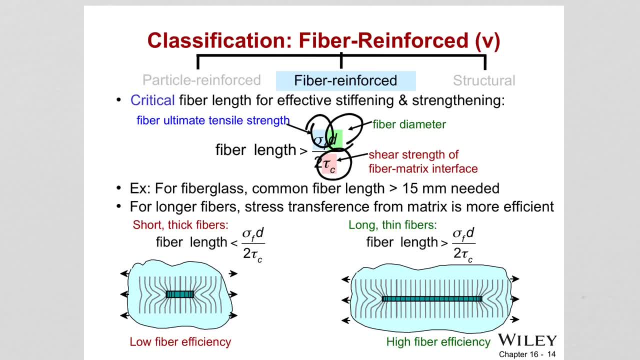 to transfer to the matrix. so it is. so it can use its full potential, up to 6 gigapascal, for example. okay, so for short and thick fibers you are seeing, the critical fiber length is below the fiber length itself. I'm sorry. the fiber length itself is below the critical fiber length, right? so L is when it's smaller than. 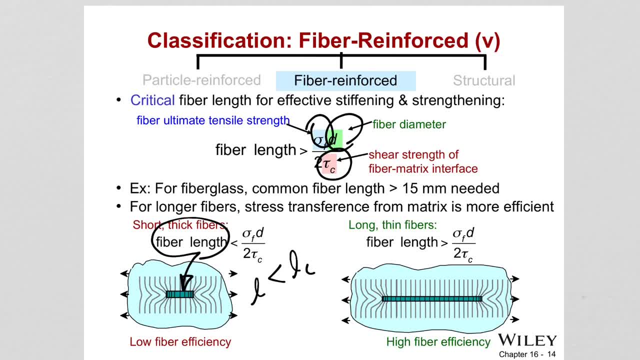 critical fiber length, you have low fiber efficiency, meaning you are not using the full potential of the fiber. you are not transferring all stresses efficiently to the fiber. so length really is important. okay, but there is this in this figure: the stress distribution around the fibers are given to us. 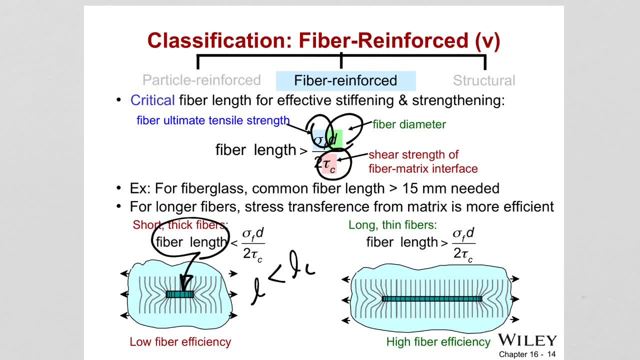 so, in other words, we can show it in a graph. okay. so in the y-axis we can have stress and in the x-axis it is the position 0 from 0 position of the fiber to it if it's length L up to size L. okay, 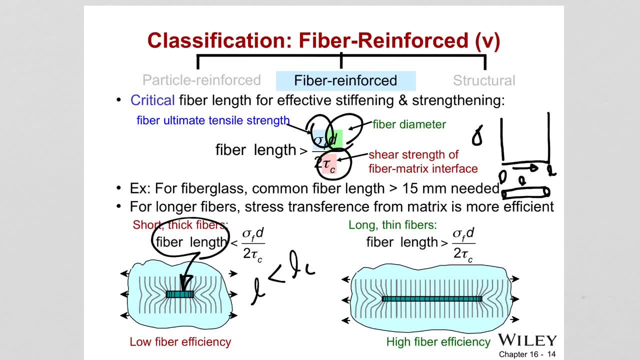 in the x-axis. so if you have fibers where L is lower than the critical fiber length and the stresses distribution, the fiber experiences looks like this. so it means that the maximum stresses are experienced in the middle, actually, and at the edges it is lower. so your fiber strength is right there. okay, so you are not actually achieving an efficient transfer. 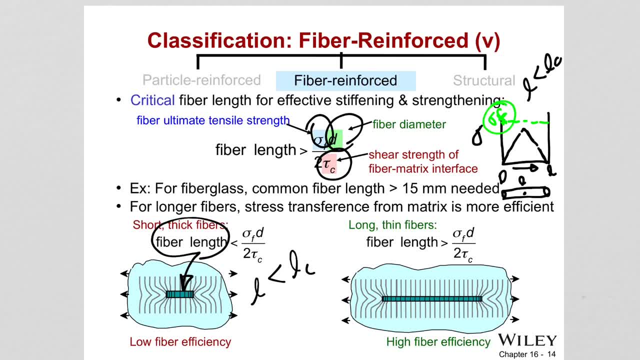 of stress you are not achieve using the full potential of the fiber itself. fiber can handle more stresses, but this is the maximum it is handling right now. it can handle more, so you should efficiently transfer the stress. but if this is also other way around is also possible when you have fibers that are that fiber. 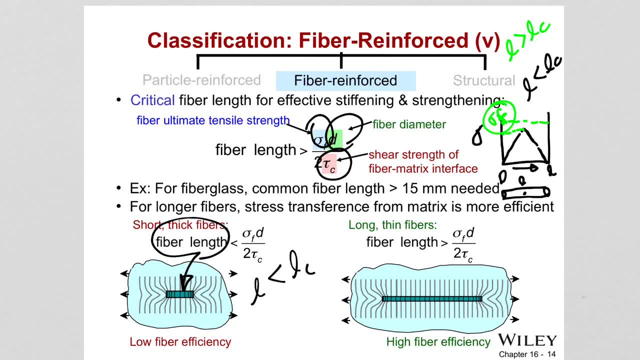 size is bigger than the critical fiber size, then you actually reach its maximum potential and all fibers now handling stresses at their potential, at their fracture strength, failure, strength, okay. so this is the case in here. where L is bigger than Lc, it's a continuous long fibers, okay. so the key here is, in summary, that there has to be a critical 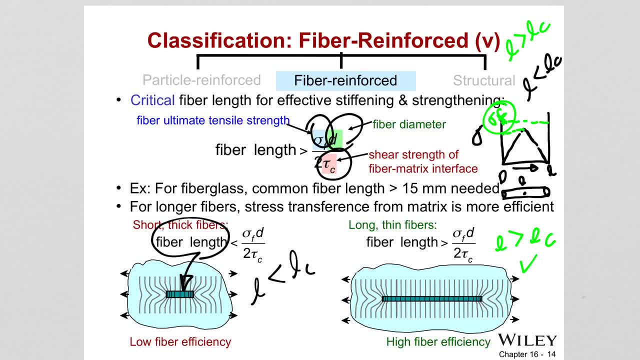 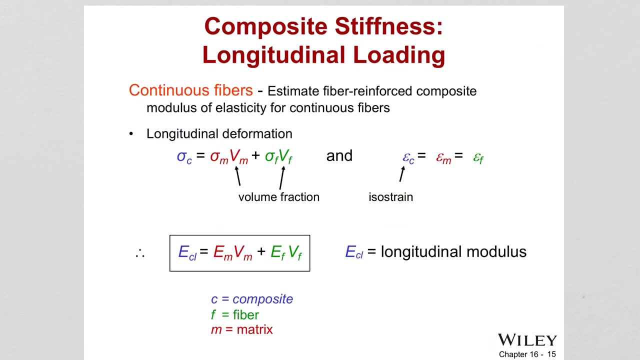 fiber length for a certain system, fiber system where it you are able to efficiently achieve strengthening and stiffening. okay, because this and also this critical fiber length depends on the fibers strength and then diameter and then the shear yield strength of the matrix, I mean the interface between fiber in느루 Matrix. so how do we determine the? again, the modules or properties? 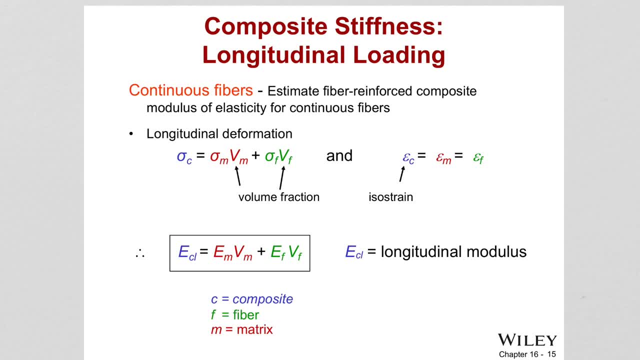 karşulü and modulus of fiber reinforced composites, and the same idea here that we have applied to particle composites is valid, which was the use of rule of mixture to equations to identify the extremes, so max and min values of stresses and moduluses that can that the composite can get, so when stress is. 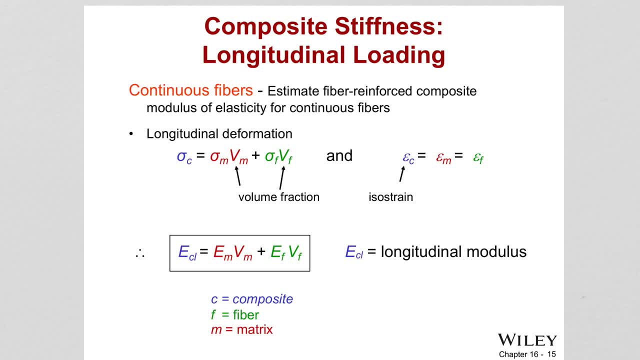 applied parallel to the direction of fibers, which means longitudinal loading. okay, so you have fibers like this and stress is applied parallel to that, longitudinal, so the deformation of both matrix and fibers is the same. when this is the case, we call it isostrain state. isostrain state means longitudinal modulus, so 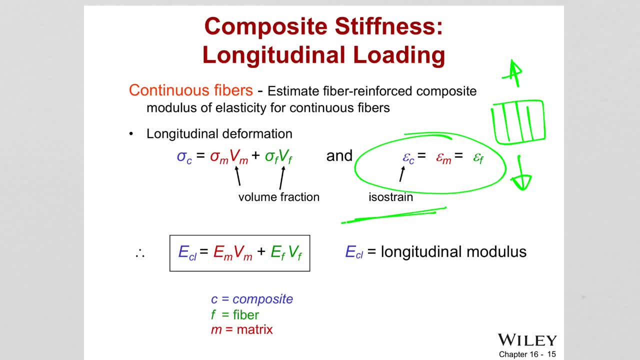 isostrain means that the deformation of the matrix, strain of the matrix and the fibers are the same and is equal to the overall deformation of the composite. and when? when this is the case, equations can be derived and we're not going to go into the derivation but, again, using the rule of mixtures we can able to identify. 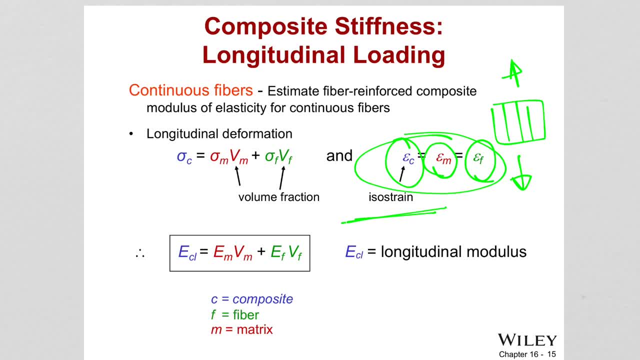 the strength of the composite and modulus of the composite. in longitudinal, the direction L means accompany to L and C means the composite and L means the log. and you see it depends on the volume fractional, again right: volume fraction of the matrixes and volume fraction of the fibers. in this case 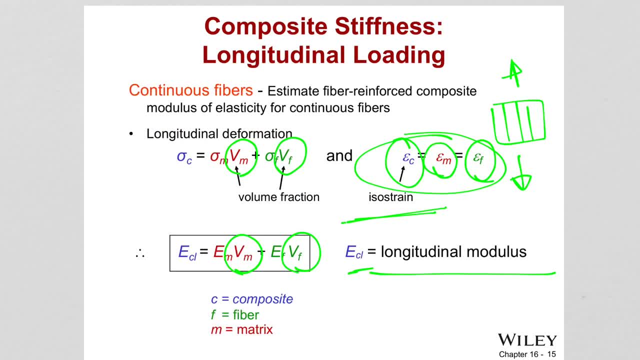 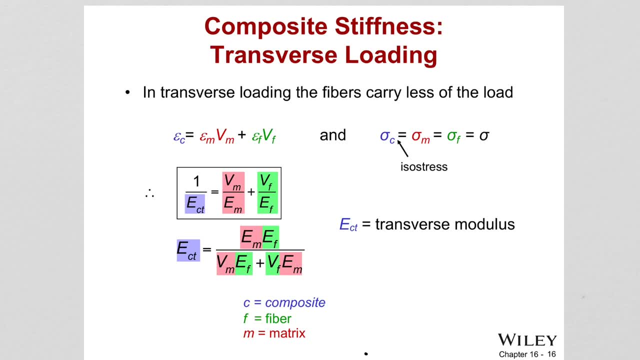 so in transfers, loading, the means in this transfers direction, if you load, how can we calculate the modulus or stress? so in the load is applied at a 90 degree angle to the direction of fiber alignment. in this case stresses, not strains, in two components are equal. you see how it is expressed. okay, in that case, with. 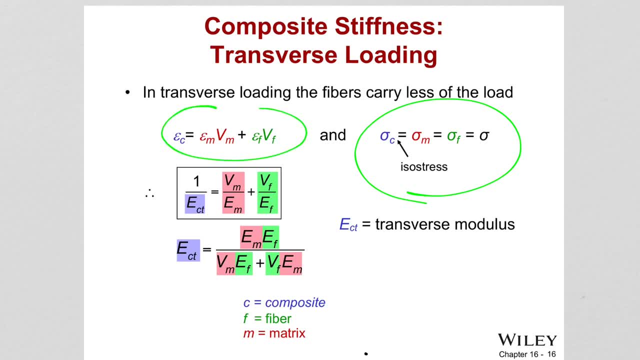 this knowledge that the composition deformation also depends on the volume fractions. based on these equations, equations for the modulus can be derived. again, I'm not going to the innovations, but here you can see the final version of the how we calculate actually the modulus of the composite. and this is the same equation written in a different version. it's the same thing, basically. 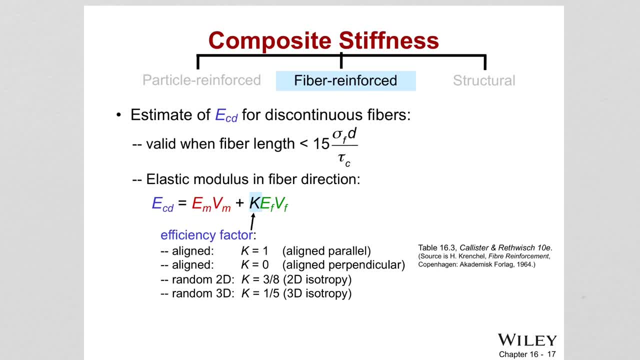 okay. so there are other equations have been derived. for example, what if the fibers are discontinuous? how we can estimate the stiffness or the Young's modulus when this is the case and this equations, are we going to learn a valid only 15 times of the critical fiber length equation? and 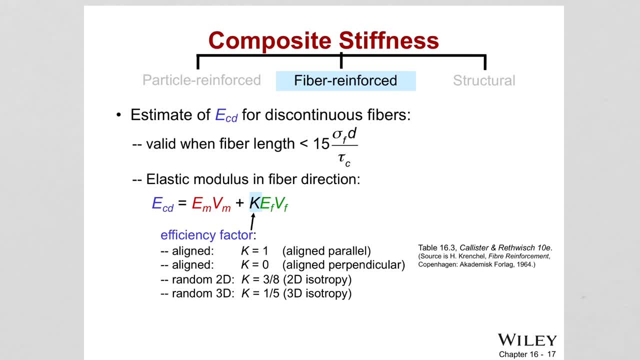 so in this case elastic modulus, how we calculate in the fiber direction. here you see the same equation here we are using, but it now includes an efficiency factor and, if it's aligned, an efficiency factor K. if aligned, this efficiency factor K is 1. if not aligned, made it the perpendicular efficiency factor 0. that makes no. 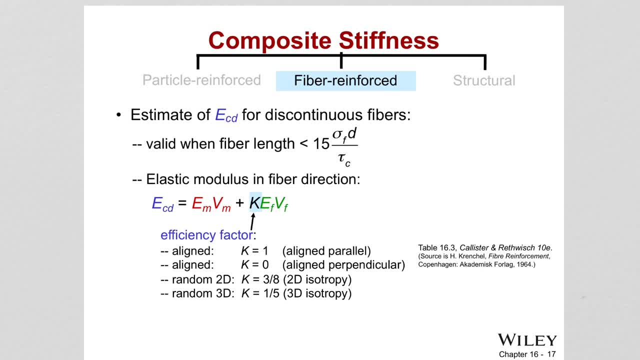 effect of fiber in the modulus right, because if you put 0 to k that makes this term zero. therefore the effect of fiber. there is no effect, pretty much right. so that is how alignment is important. random arrangement in 2d and 3d you achieve different isotropy and it is the k factor just changes and depending on that you can calculate. 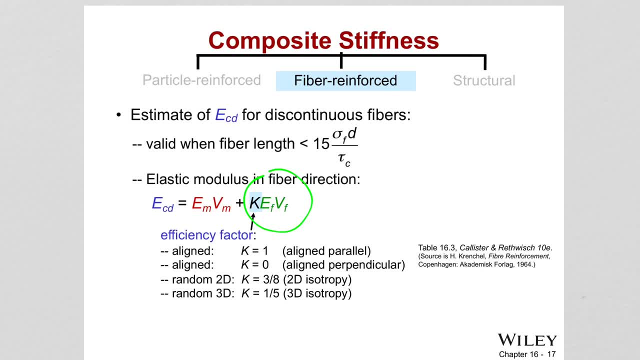 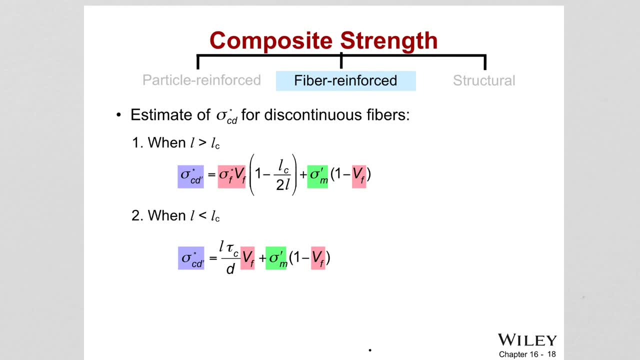 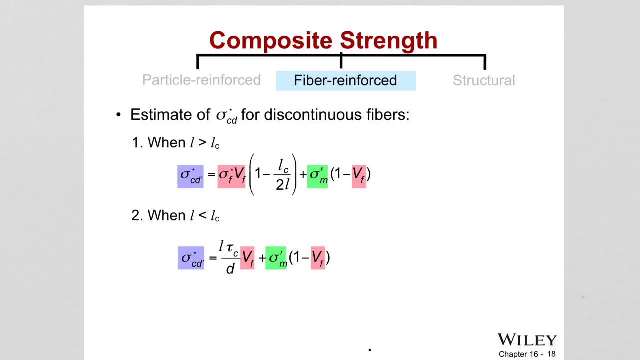 going to use depends on if you have lengths bigger than critical length, critical fiber length or smaller than critical fiber length. So based on that, you see, different equations are given to us which are basically much developed experimentally. that gives us what type of stress levels we expect from a. 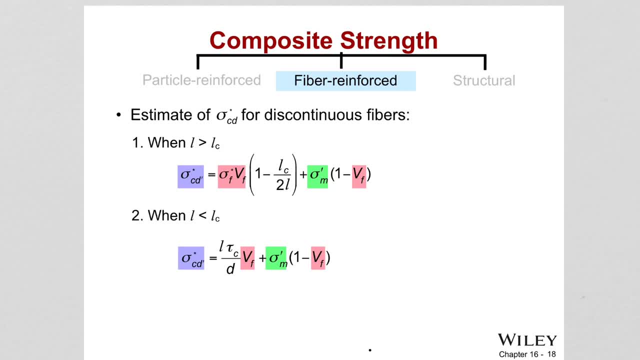 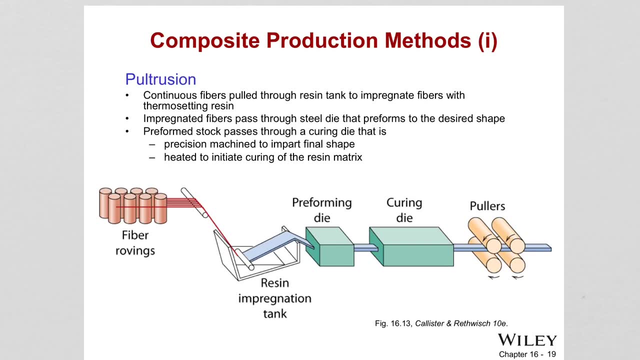 composite if it does have discontinuous fibers. Now, finally, we're going to take a look at composite production methods. so how do we produce composites? So one example is pultrusion. Here we have continuous fibers. this is an example of a polymer matrix. okay, polymer matrix. 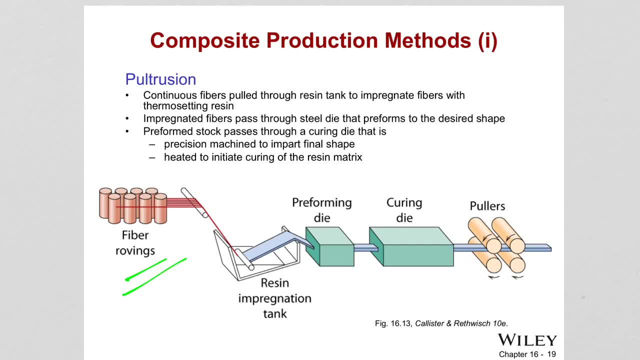 fibrillation, which is a principle that we refer to as the reinforced polymer matrix composites. here the continuous fibers are pulled through a resin tank to impregnate fibers with thermosetting resins. so first the fibers are quoted with the resin. okay, and this is thermoset, Thermoset. remember, thermosets are the 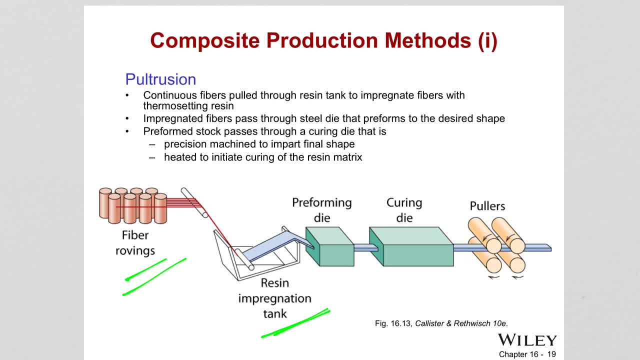 ones where you have covalent bonding between the chains like that. okay, so a. But before these covalent bonds between the chains form, first you impregnate the fibers with the resin. You are not doing the curing. Curing means that you are actually forming these intermolecular or the bondings- covalent bondings in between the chains. 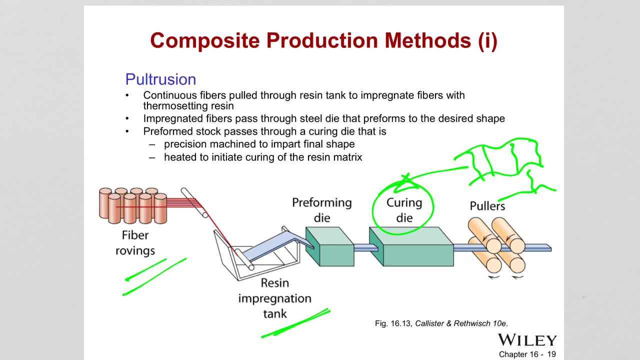 You are forming it at this stage. You don't want to form it initially because then you cannot. they are not, you know it doesn't have a viscosity. it is pretty hard material if that does happen. So first you impregnate the fibers, then it goes through preforming dyes to preform to the desired shape. 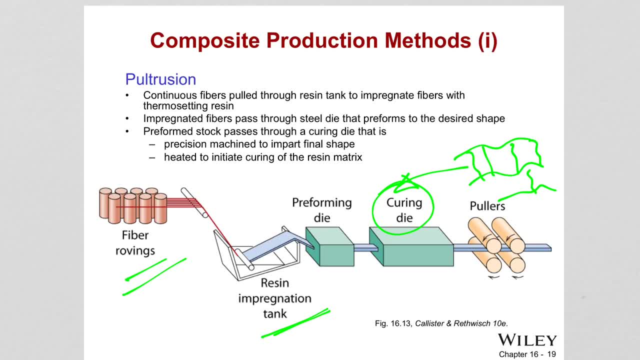 After the preform you are going to do the curing. After the preform the stock passes through a curing dye, it goes to pullers, where it is machined into a final shape and at the same time heated in to initiate the curing here of the resin matrix. 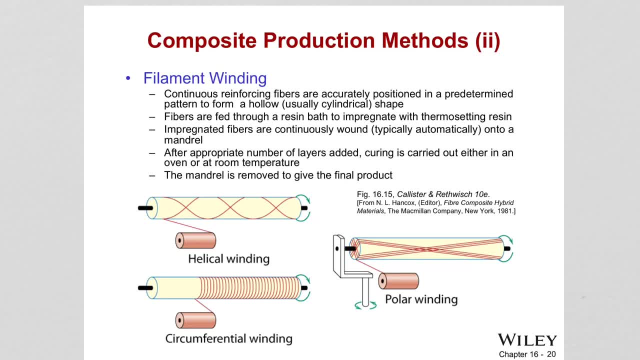 Then there is filament winding, and this is used, for example, in the formation of the chains, The construction of vaulting poles. See, here you have a continuous reinforcing fibers, like here. And then what is happening here is the fibers are positioned in a predetermined pattern to follow a hollow shape. 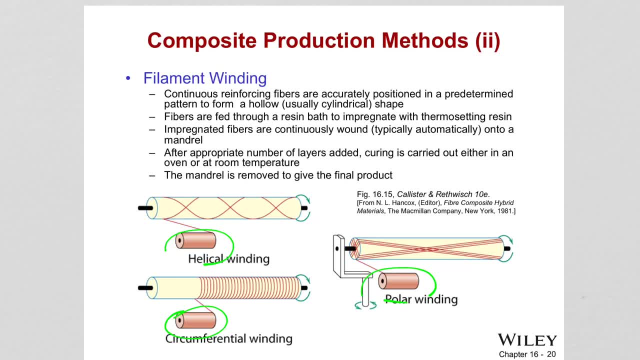 So the filament winding technique is to make hollow shape composites. Fibers are first went through a resin bath to impregnate again with thermosetting resin. So this is how they introduced the matrix. okay, They caught the fibers with the resin first and then this impregnated fibers then continuously wound onto the mandrel. 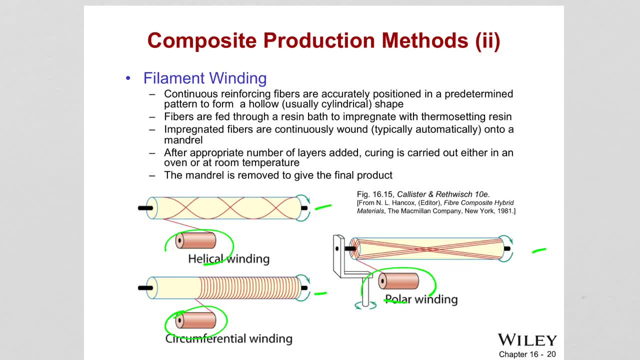 You are seeing the mandrel different type. okay, I mean the mandrel is a different type of winding is happening: helical Or circumferential or polar. So after appropriate number of layers are added, curing is carried out either on an oven or at room temperature. 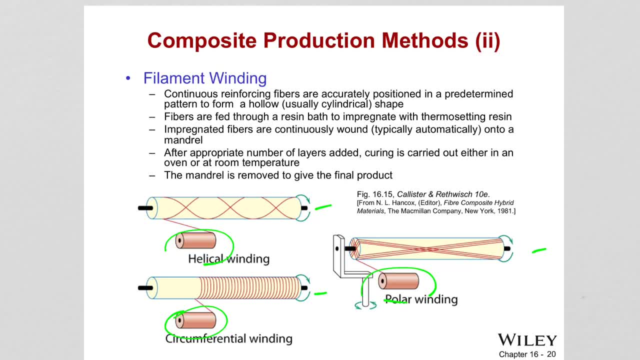 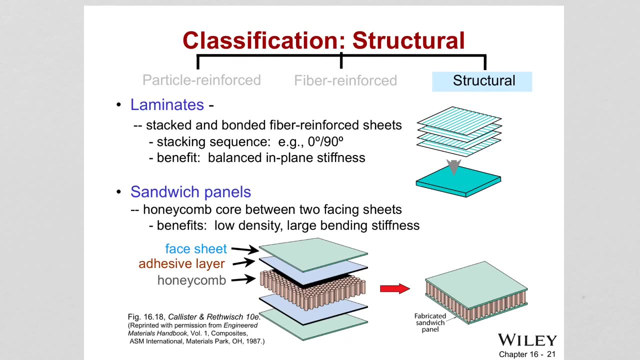 Then the mandrel is removed, which will give you the final product, And I suggest you guys, you can watch the videos I am sending you to if you are interested in how this process looks like. So structural one, So structural one, So structural one. 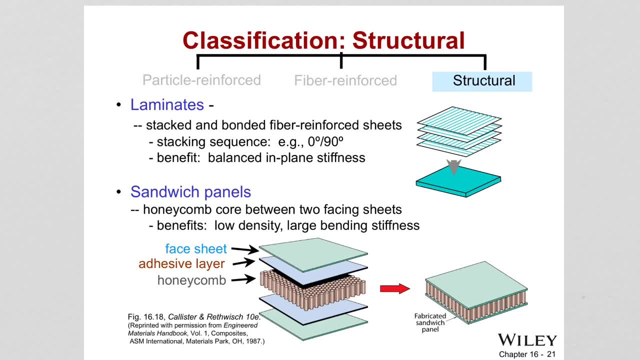 So structural ones are laminates and sandwich panels. So you are seeing different sheets of fiber reinforced components In which each of these fibers are aligned in a different direction. We call it this: changing from zero degree to 90 degree alignment. Ok, so here is individual sheets. here you achieve only strengthening in one direction. 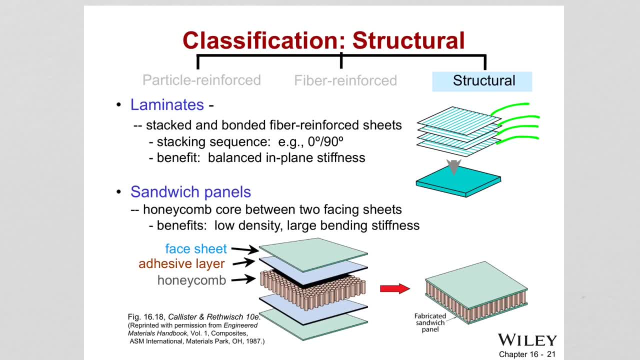 But if you stack different layers, that the fibers align in different directions, then you can achieve stiffness in all directions. right? This is the idea of the laminates. You stack them together, stack the sheets And sandwich panels. you see, this is like a honeycomb structure. 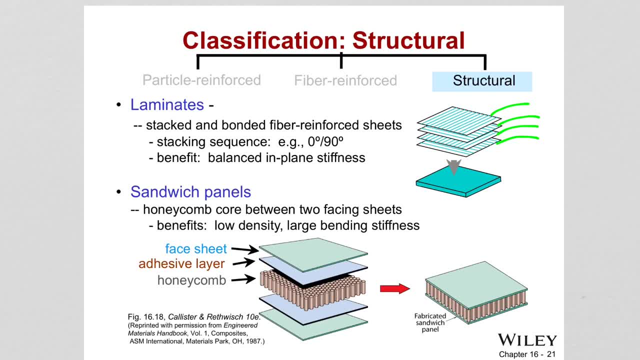 usually a honeycomb core between two facing sheets. This will have a low density and large bending stiffness. As you see that the shaping, giving the material different shapes, even that can change the stiffness of the materials. So, playing with the different wide range of materials and also changing the shape, 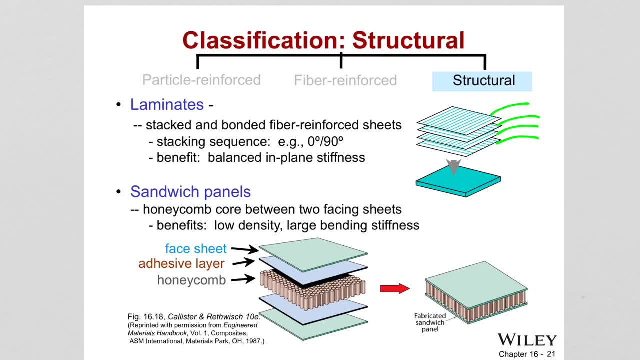 or putting together different shapes of layers, also changing the properties, And it depends on actually what type of properties you desire, And in this case with the honeycomb structure, which is usually desired to be used in aerospace industry. it has low density but high, large bending stiffness. 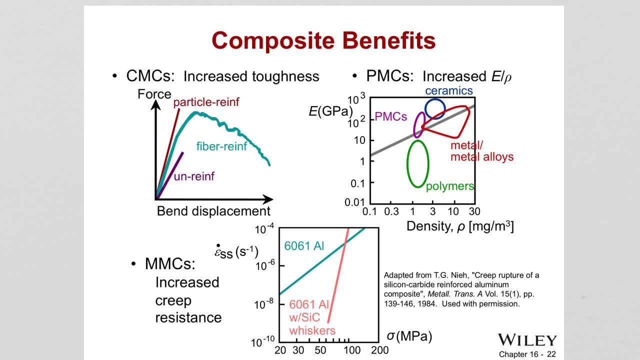 So, if we want to summarize, what are the benefits of composites? If you have a ceramic matrix composite, you are increasing the toughness. okay, So you are measuring properties. If you have a christian ceramic crochet and you have diss� 씨? 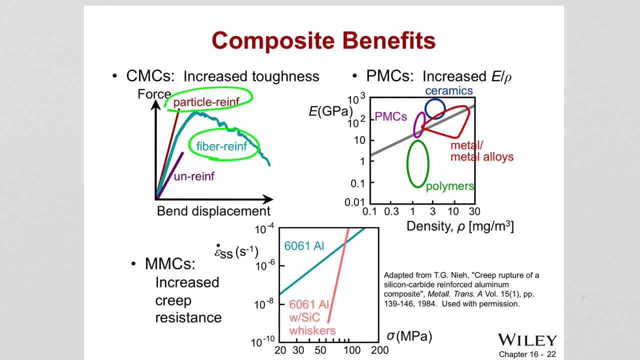 And we mean to say theоч, e think formal ceramic. So you canачiy. Oh the common. sorry, What's the common? The common principle, The common principle is a common principle, right. The common principle is that the common principle is very important for shampooing. If you can't see it right, you can't see it. So you can't see it, Not because you are not very careful, you do the fact. What do you mean? if it's difficult, You might be very careful. So the common principle: even with the manufacturing process, you can see a little bit more. 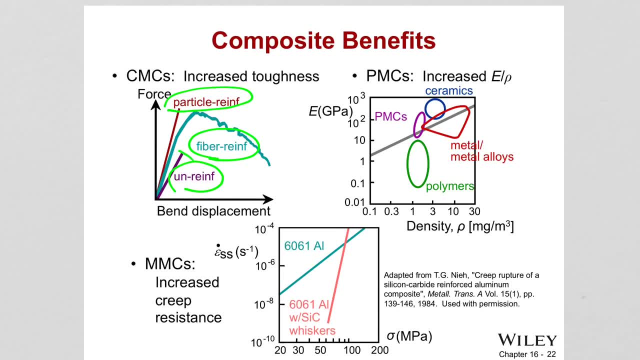 It just takes some time to know what the picture is about And just like doing just anything you can like. you see, it fractures right right there, at low forces, at low stress levels. but putting a fiber it gives it some plastic deformation, some higher strength values. so it is actually, you see. 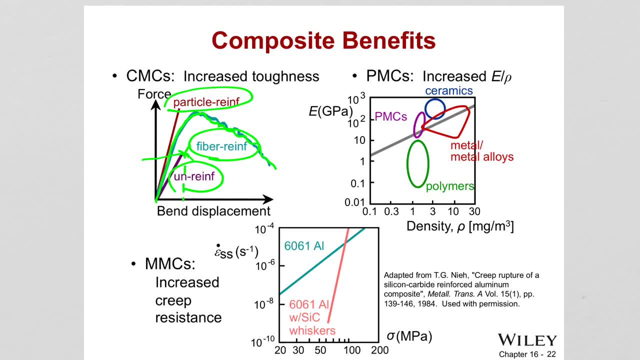 increasing the ductility because it breaks right there. but this breaks right there, so it is increasing the ductility and toughness, toughness, the area under the stress strain curve. and then what about the polymer matrix composites? so the idea here is: polymers are not strong, the 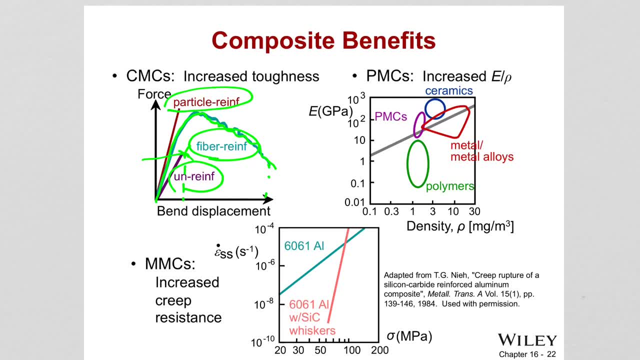 whole idea is, polymers are lightweight but they are not strong. so if i put some certain fibers or reinforcements i can get something that is low weight and increased stiffness and strength. in other words, i can increase specific stiffness, which is the modulus over density i can increase. 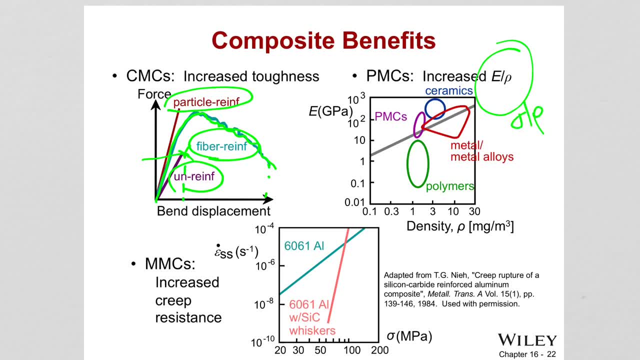 that or specific strength. okay, and as you are seeing that the density of polymers are low here compared to other metals, metals and ceramics materials, and that is the whole idea is to basically and just enhance their keep that density but then enhance their modulus level by just making them into composite form and metal matrix composites. the idea here is: 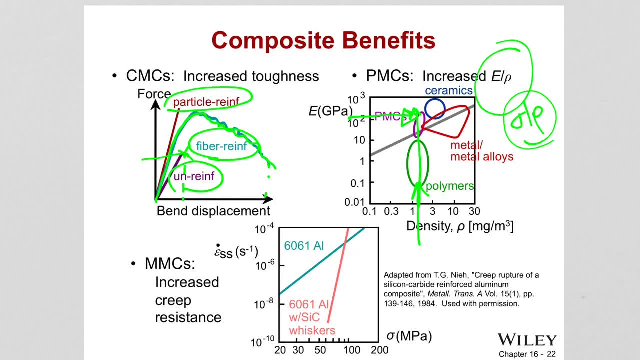 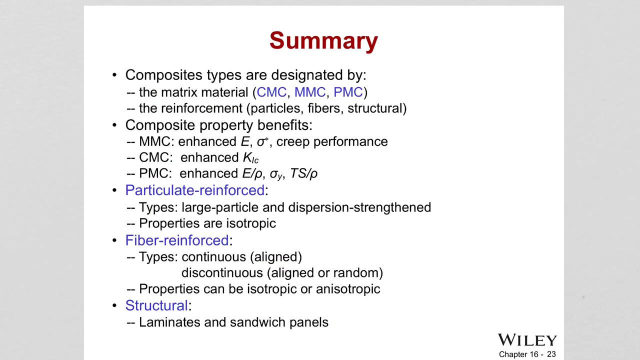 to increase the creep resistance of metals. so you see for a certain strength, strength volume. you see that when you have a metal matrix composite, its creep rate is smaller compared to the one that is just pure aluminum alloy without any silicon carbide whiskers in it. In summary, we have learned: you can have. 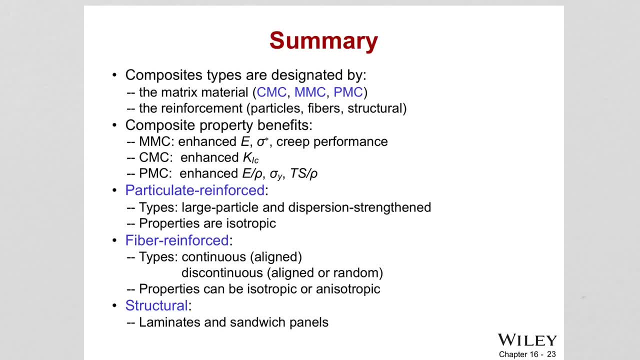 different types of composites. It depends on what type of matrix material you have. It can have ceramic matrix, metal matrix, polymer matrix. Reinforcements can be particles, fibrous, structural, And for different composites goals are different. In metal matrix, you want to achieve better creep performance. In ceramic,